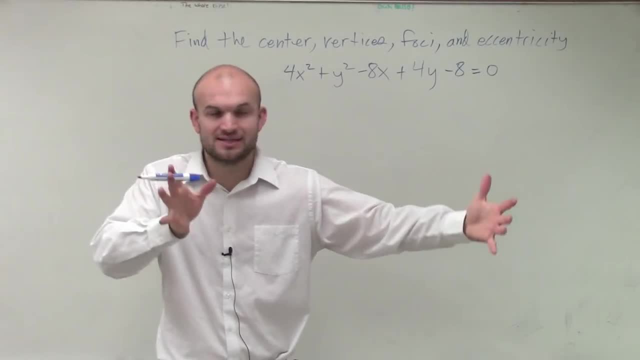 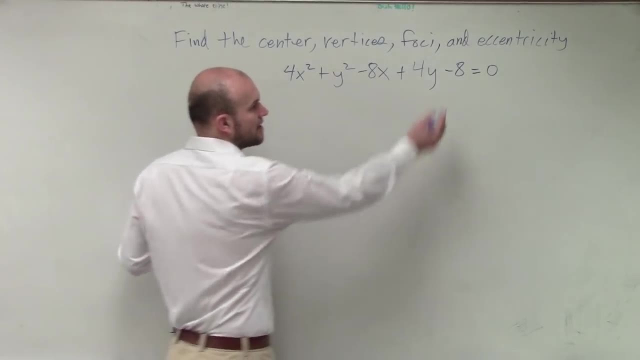 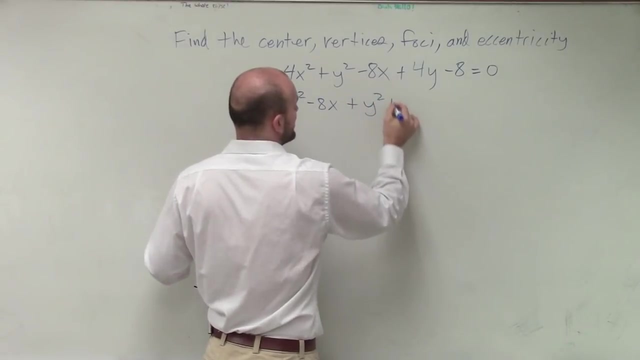 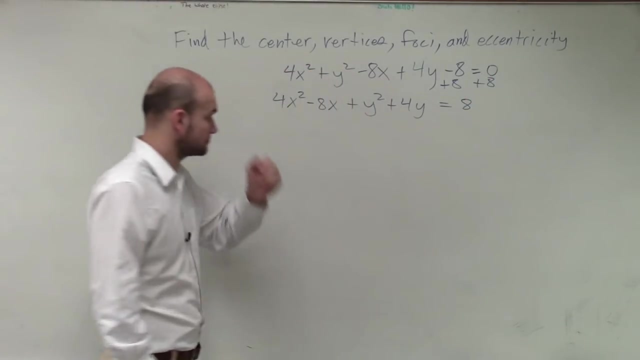 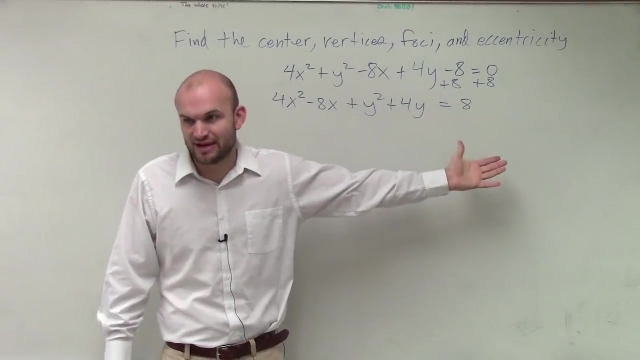 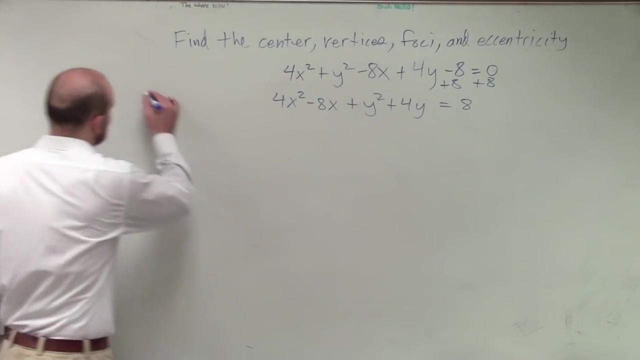 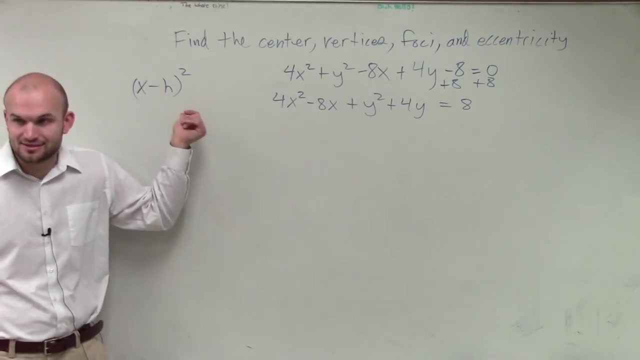 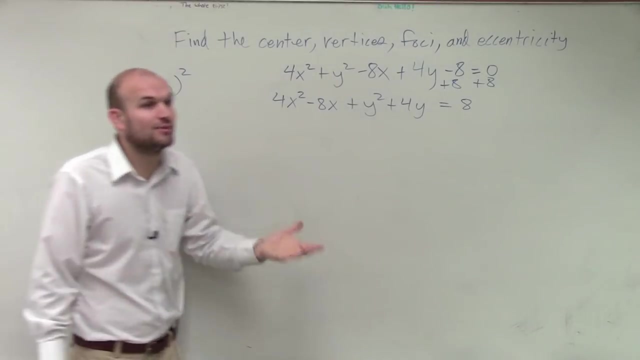 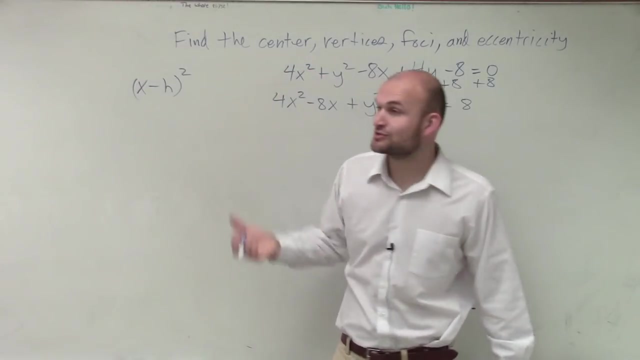 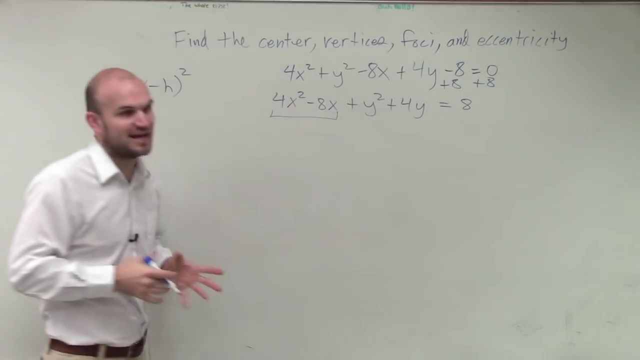 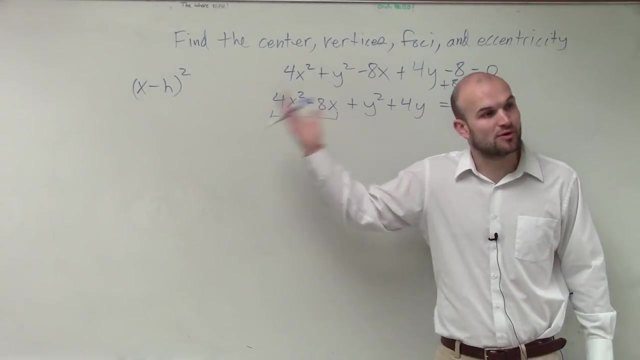 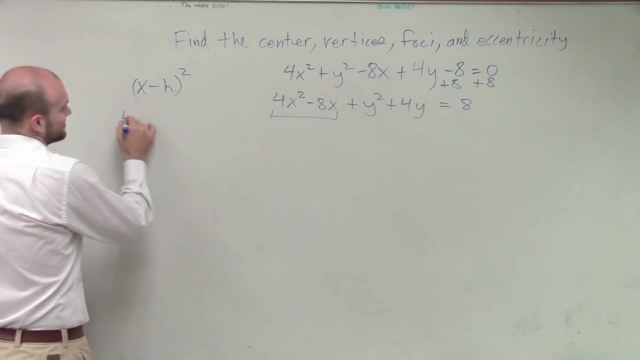 Right? X plus the Y. It was X minus H squared and then plus Y minus K squared. So what I'm going to first do is let's group the X's and the Y's. And then I'll get that constant over there. So I have 4X squared minus 8X plus Y squared plus 4Y. And let's add the 8 to the other side. Okay? Now, it looks a little bit closer. We have the X's. We have the Y's. And we have an 8. However, that wasn't the formula, right? It was supposed to be X minus a number. So I need to get this, X minus H squared. I need these X's to look like this. Right? This to look like that. Correct? Right. And the only way we can do that is what this is is, remember, this is a binomial square. A binomial square. The only way we get a binomial square is by adding the X's and the Y's. So what we're going to do is we're going to factor a perfect square trinomial. So I need to take this and make it a perfect square trinomial. And the only way that we've learned how to make a binomial into a perfect square trinomial is by completing the square. So to do that, let's take it. So we have 4X squared minus 8X. I need to complete the square. I need to make this a perfect square trinomial. 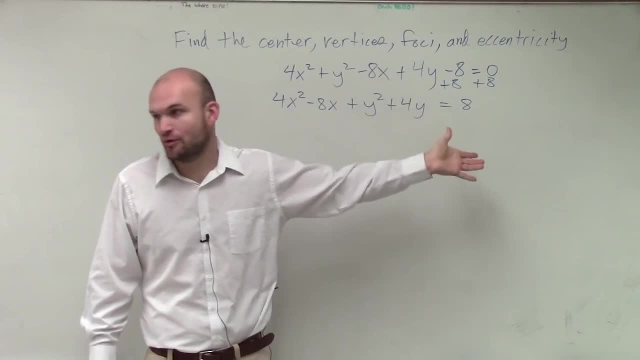 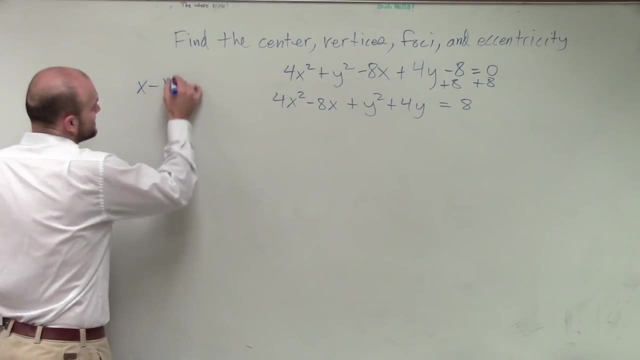 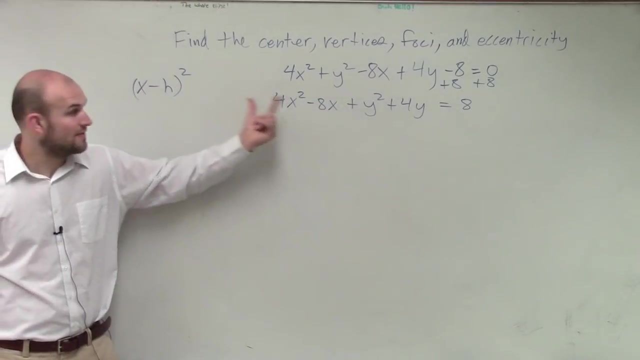 And we have an 8.. However, that wasn't the formula right. It was supposed to be X minus a number, So I need to get this X minus H squared. I need these X's to look like this Right, This to look like that Correct Right, And the only way we can do that is what this: 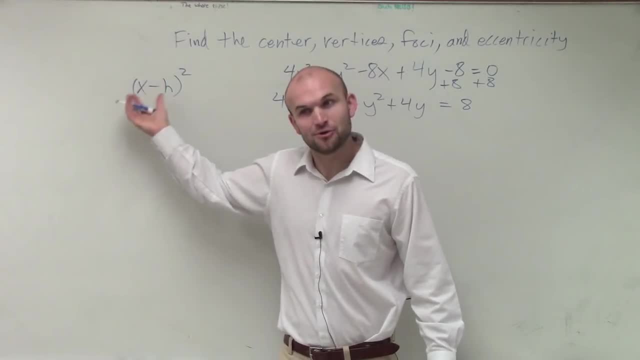 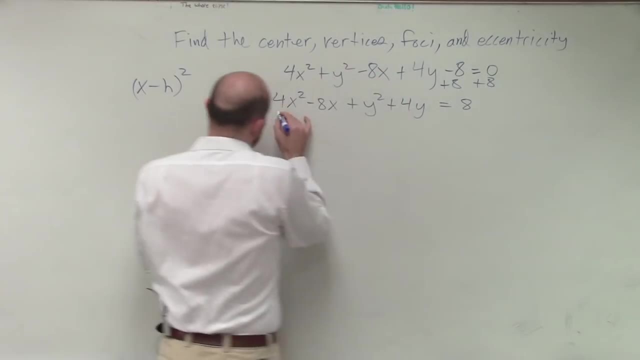 is is remember: this is a binomial square, A binomial square. The only way we get a binomial square is by adding the X's and the Y's. So what we're going to do is we're going to factor a perfect square, trinomial. So I need to take this and make it a perfect square. 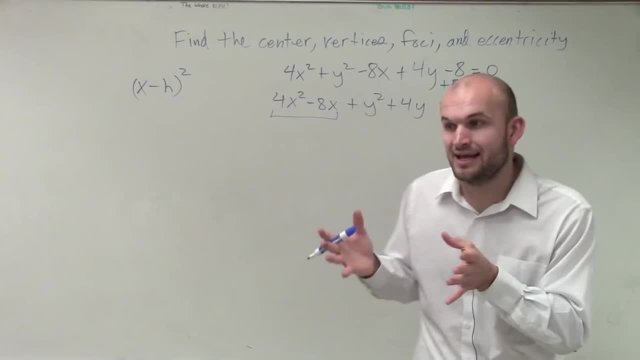 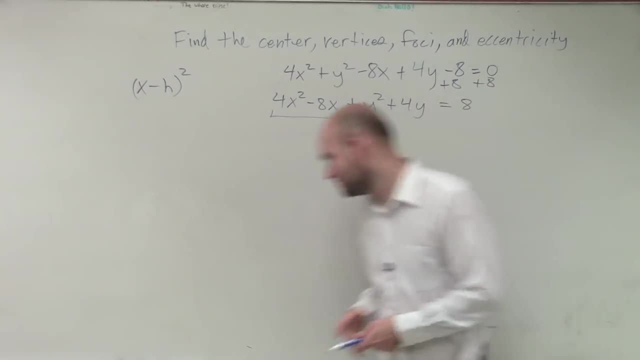 trinomial, And the only way that we've learned how to make a binomial into a perfect square trinomial is by completing the square. So to do that, let's take it So we have 4X squared minus 8X. I need to complete the square. I need to make this a perfect square trinomial. 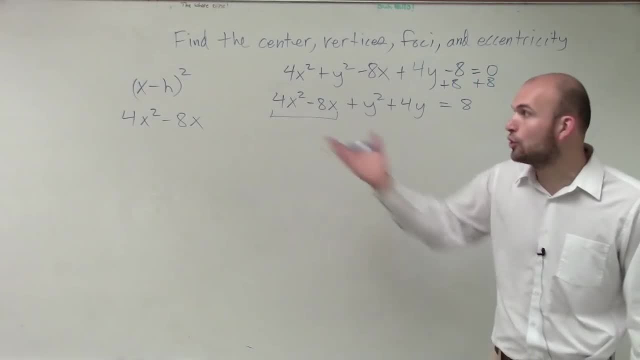 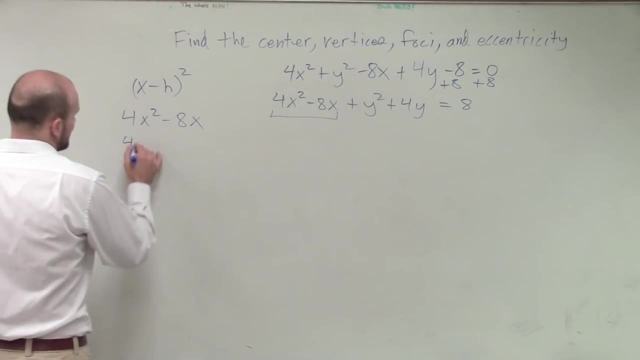 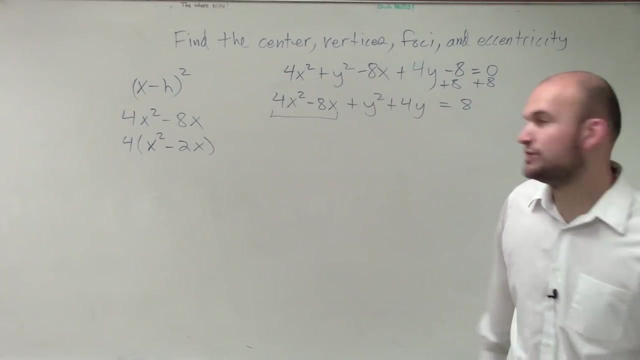 Remember, the first step in completing the square is you cannot have a coefficient of anything besides 1 in front of your quadratic term. So the first thing I do is I factor out a 4.. Right Then, remember, we do our special little case in doing D divided by. 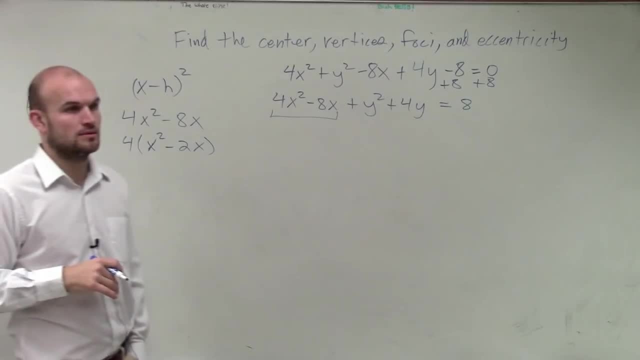 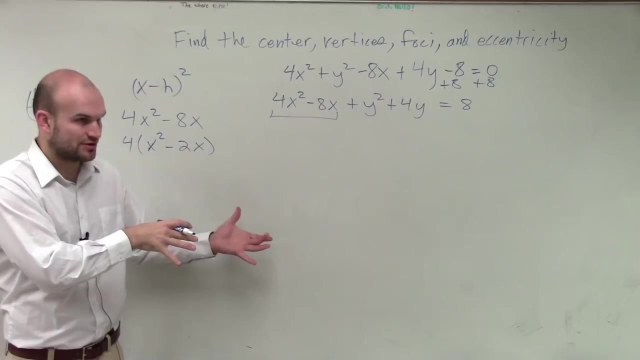 2. And square? Huh, You can but remember. we want to keep this as a quadratic. You could factor out an X, You're right. But if you factor out an X, then you're not going to remember. our whole purpose of completing the square is not to factor it, but to create. 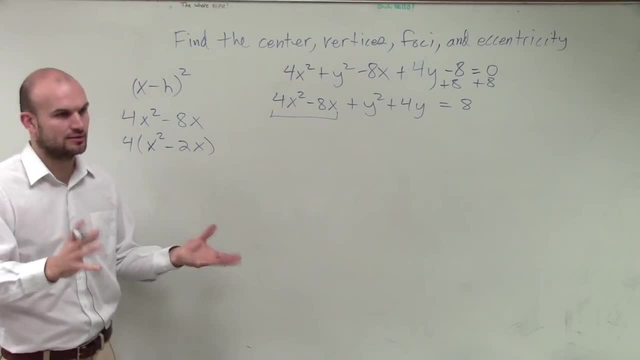 a perfect square trinomial, that's quadratic, Right. So we do B divided by 2,, which is, and then I do negative 2 divided by 2,, squared, which equals negative 1, which is 1.. Right. 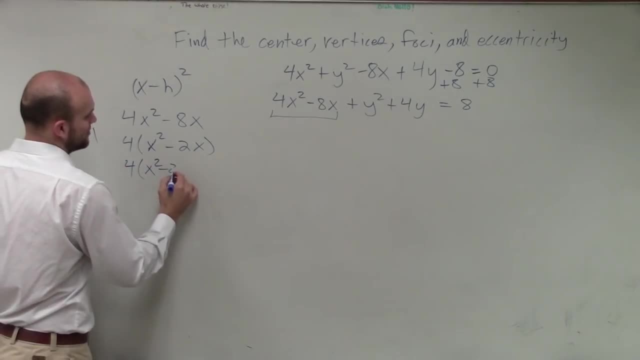 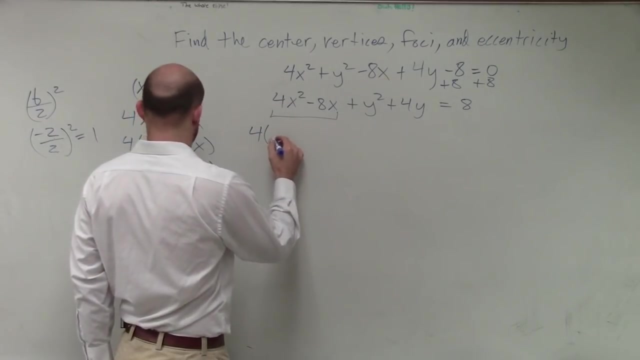 Yeah, So I have 4 times X squared minus 2X plus 1.. So let's write that in there. So I have 4 times X squared minus 2X plus 1.. But now, ladies and gentlemen, remember whatever. 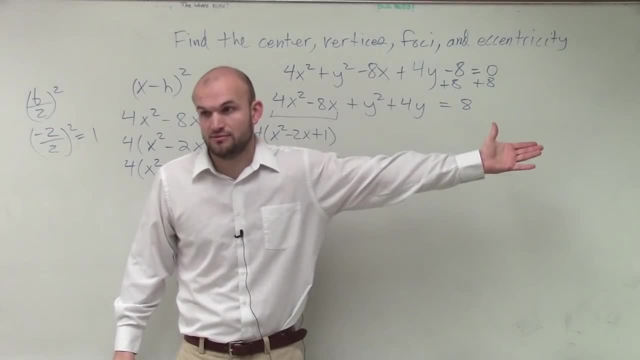 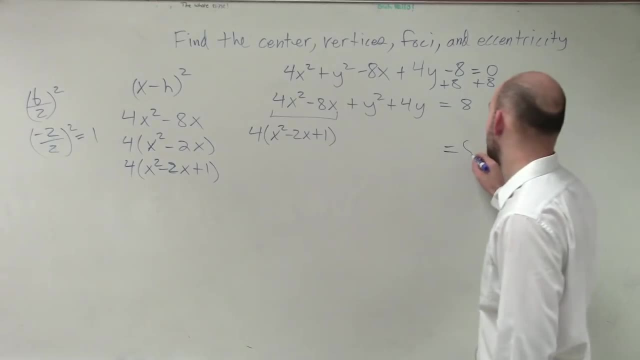 we do on one side, we always have to do on the other side. Right Now, what am I actually? what did I do? What did I actually add to this right side? 4.? 4. Right, Because I added a 1.. So from here, 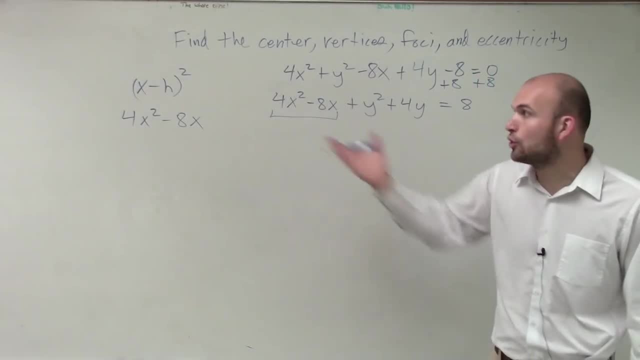 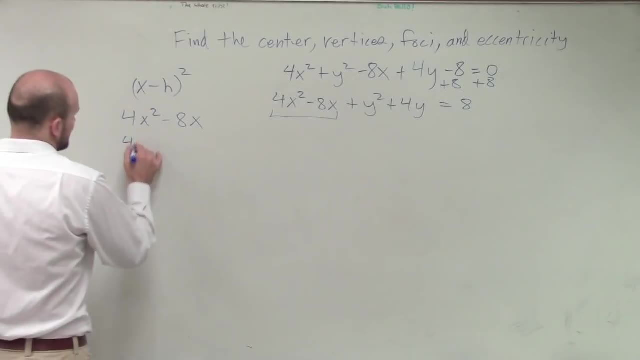 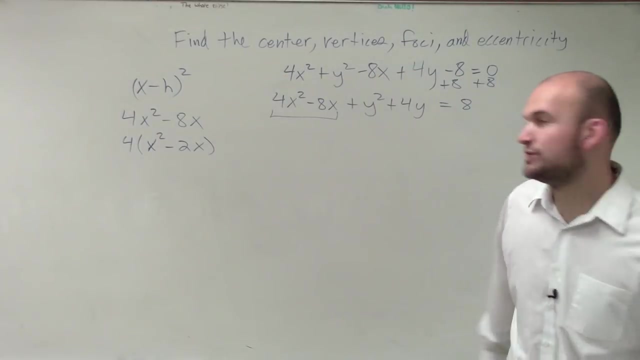 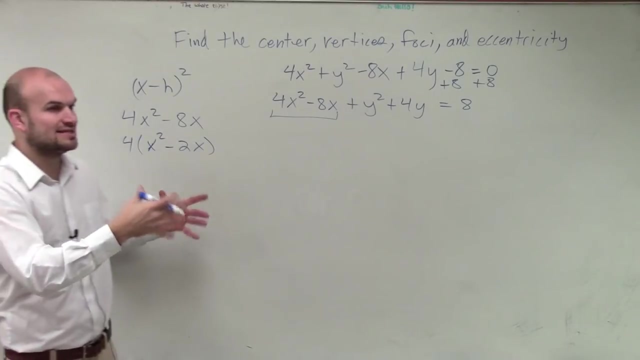 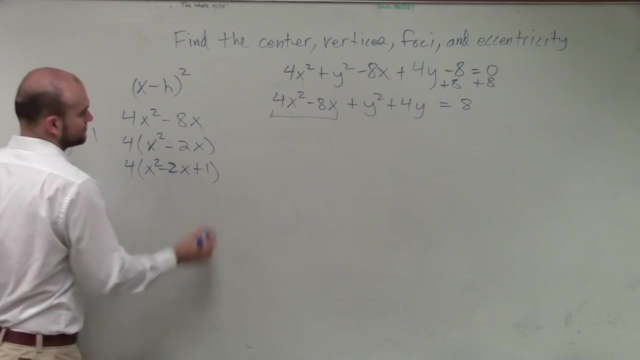 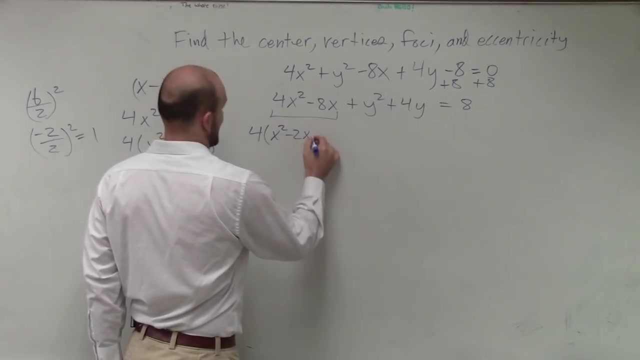 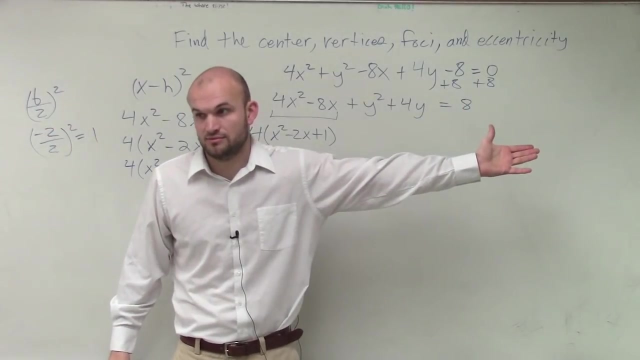 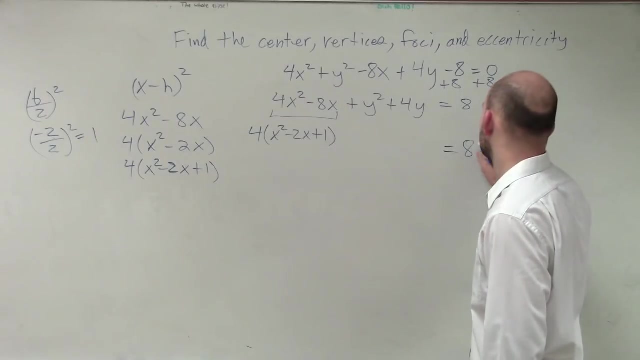 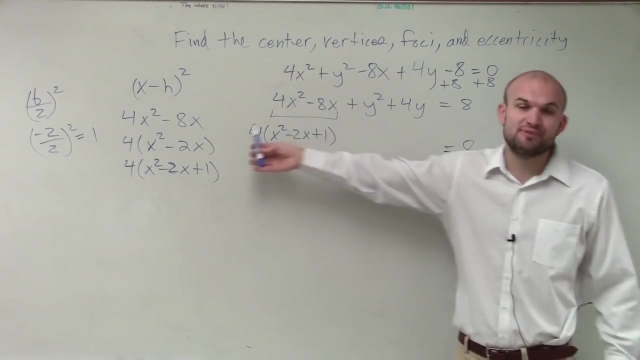 Remember, the first step in completing the square is you cannot have a coefficient of anything besides 1 in front of your quadratic term. So the first thing I do is I factor out a 4. Right? Then, remember, we do our special little case in doing D divided by 2. And square. Huh? You can, but remember, we want to keep this as a quadratic. You could factor out an X. You're right. But if you factor out an X, then you're not going to remember our whole purpose of completing the square is not to factor it, but to create a perfect square trinomial that's quadratic. Right? So we do B divided by 2, which is, and then I do negative 2 divided by 2, squared, which equals negative 1, which is 1. Right? Yeah. So I have 4 times X squared minus 2X plus 1. So let's write that in there. So I have 4 times X squared minus 2X plus 1. But now, ladies and gentlemen, remember, whatever we do on one side, we always have to do on the other side. Right? Now, what am I actually, what did I do? What did I actually add to this right side? 4. 4. Right? Because I added a 1. So from here to here, I added a 1, but that 1 is being multiplied by 4. So over here, I'm also going to have to make sure I add 4. Right? So I'm going to have to make sure I add 4. Right? 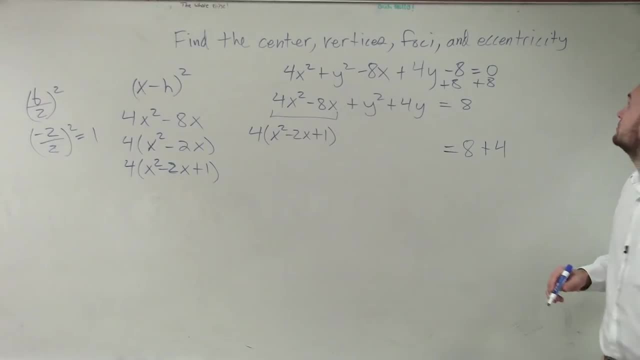 So I'm going to have to make sure I add 4. Right? So I'm going to have to make sure I add 4. Right? Do you understand from this step to this step, what's the only difference? I added a 1. Right? Well, this is factored down to a trinomial, but I added a 1. Okay? And by adding that 1, but that 1 is being multiplied by 4, outside the parentheses. So then if I need to multiply it over here. Now, let's go ahead and do the other one. The other one is Y minus K squared. Well, in this example, I have Y squared minus 2X squared minus 4Y. I need to create this to be a perfect square trinomial. So I do negative 4 divided by 2 squared, which equals 4. So now I'm just going to add 4 to both sides. Wait, why is it negative 4? I mean, I know it doesn't really matter. 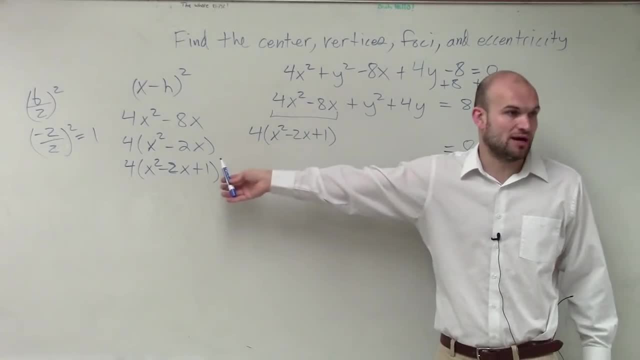 to here. I added a 1, but that 1 is being multiplied by 4. So over here I'm also going to have to make sure I add 4. Right, So I'm going to have to make sure I add 4. Right. 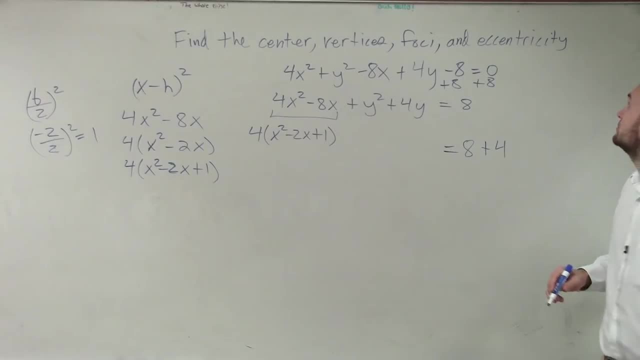 So I'm going to have to make sure I add 4. Right. So I'm going to have to make sure I add 4. Right. Do you understand, from this step to this step, what's the only difference? I added a 1. Right. Well, this is factored down to a trinomial, but I added a 1. Okay. 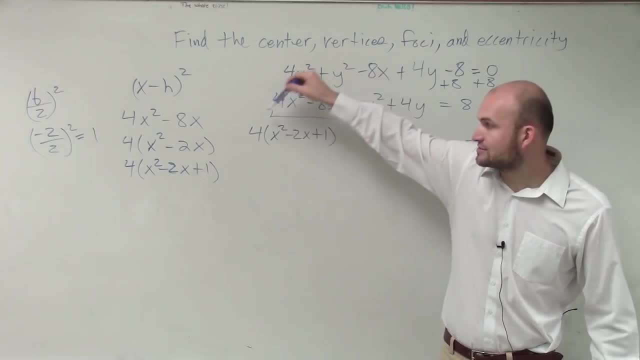 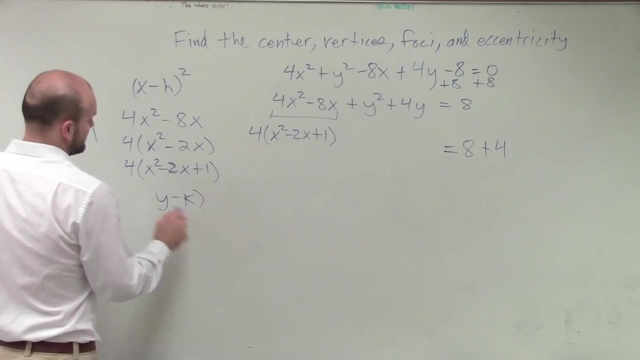 And by adding that 1, but that 1 is being multiplied by 4, outside the parentheses. So then, if I need to multiply it over here Now, let's go ahead and do the other one. The other one is Y minus K squared. Well, in this example I have Y squared minus 2X. 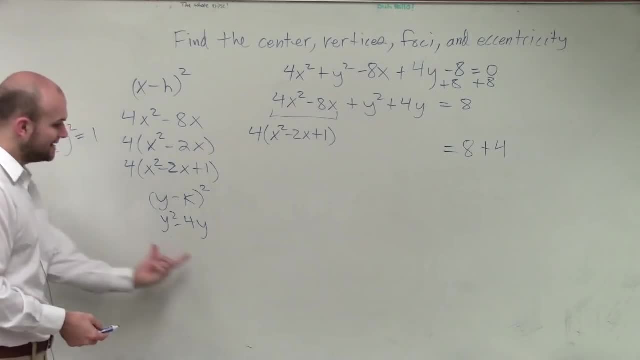 squared minus 4Y. I need to create this to be a perfect square trinomial, So I do negative 4 divided by 2 squared, which equals 4.. So now I'm just going to add 4 to both sides. 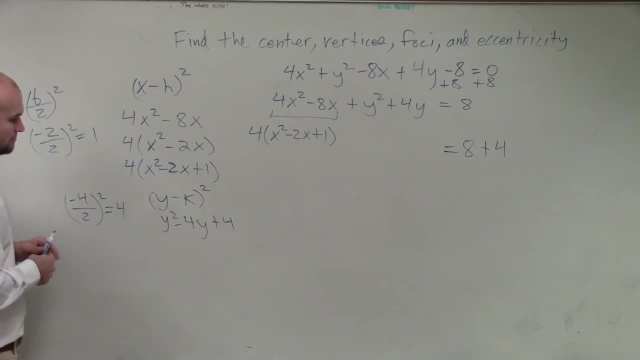 Wait, why is it negative 4?? I mean, I know it doesn't really matter. Negative 4 divided by 2 is negative 2. Negative 2 squared is positive 4.. Where did you get negative 4?? I don't know. I read it wrong. 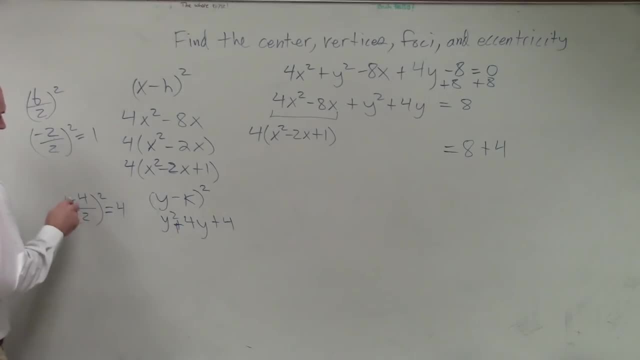 Oh, I just wrote Y last time. You're right, it's positive 4.. I didn't think it mattered. So therefore this, as a perfect square trinomial, is Y squared plus 4Y plus 4.. Now I'll keep these in parentheses, because now so somehow I added 4,, so I have to add another 4, right? 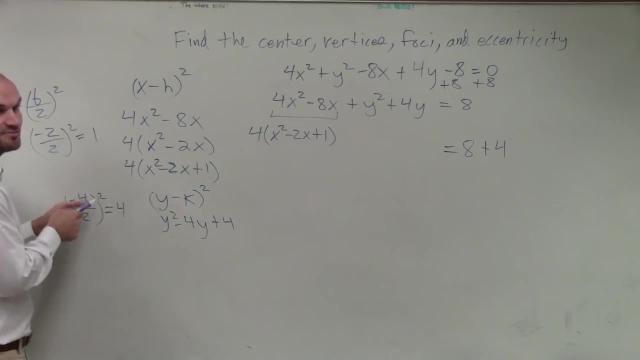 Negative 4 divided by 2 is negative 2. Negative 2 squared is positive 4. 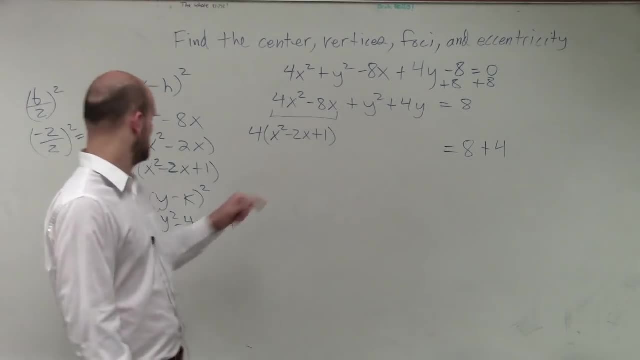 Where did you get negative 4? I don't know. I read it wrong. Oh, I just wrote Y last time. You're right, it's positive 4. I didn't think it mattered. 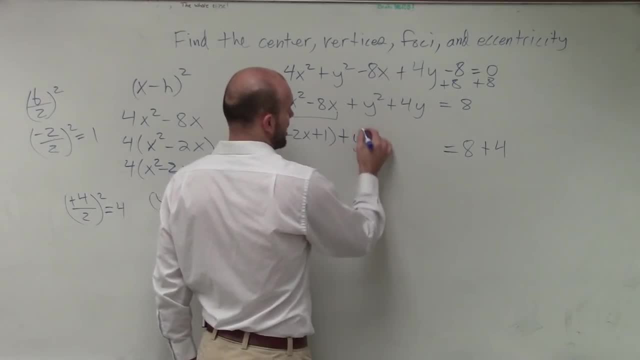 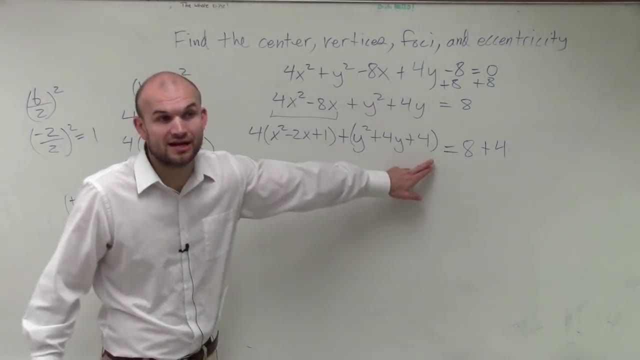 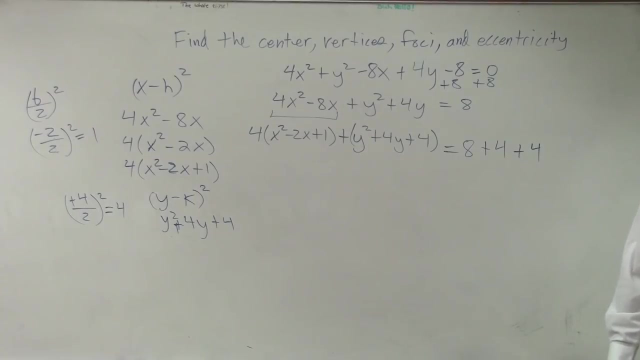 So therefore, this, as a perfect square trinomial, is Y squared plus 4Y plus 4. Now, I'll keep these in parentheses, because now, so somehow I added 4, so I have to add another 4, right? Yes? Okay. So now, why do we complete the square again? Why do we care that these are perfect square trinomials? 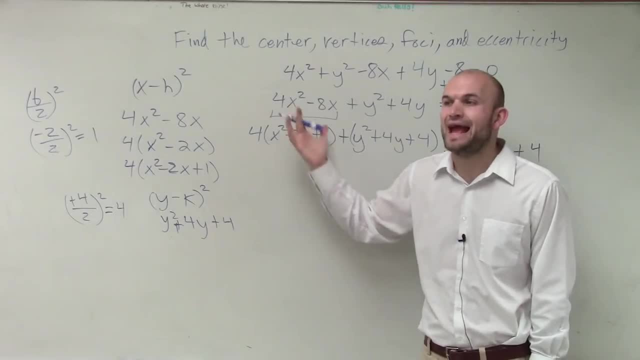 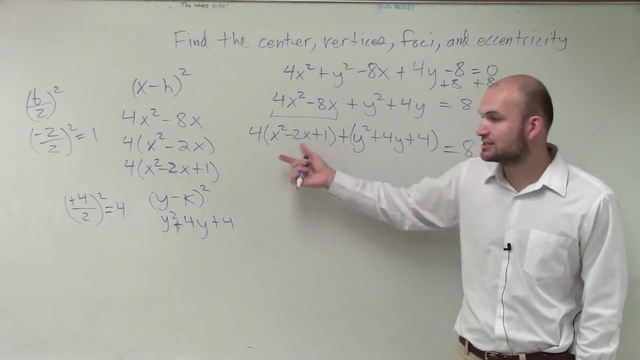 The reason why we like perfect square trinomials and the reason why we have to complete the square to create perfect square trinomials is because when we factor these, when I factor this, it creates a binomial square. 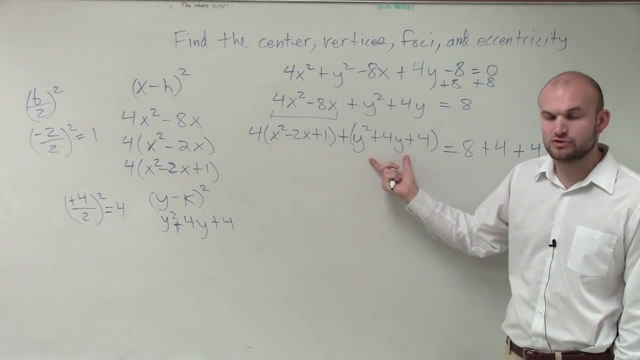 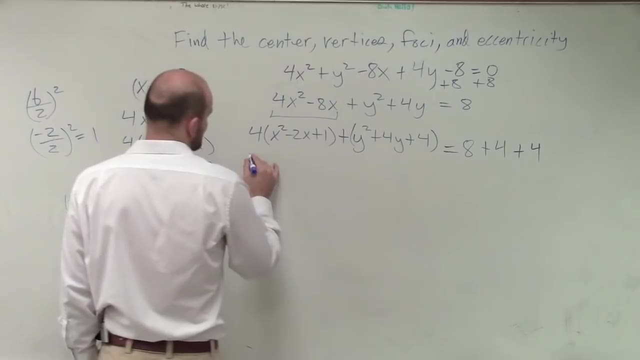 When I factor this, because I completed the square to make it a perfect square trinomial, its factored form is a binomial square. So let's go on to factor them to their binomial square. 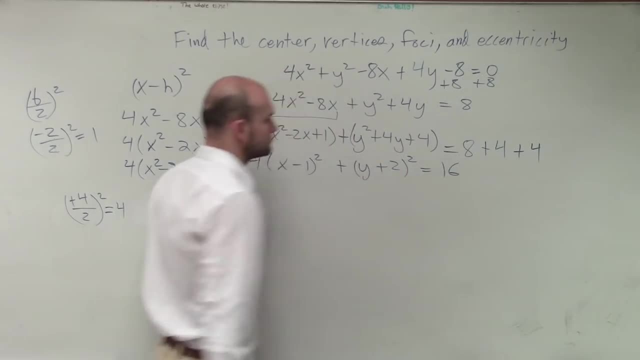 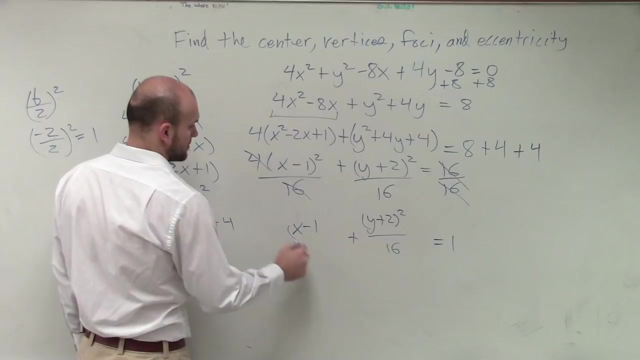 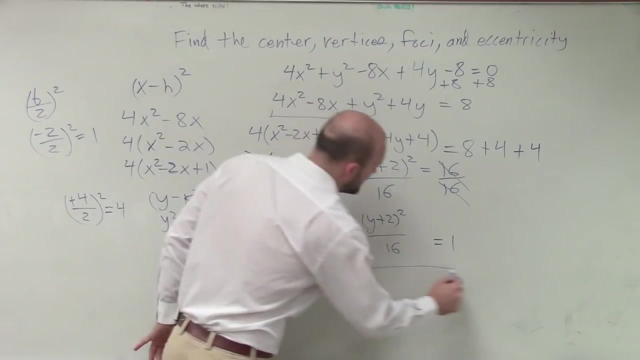 So we're almost there, right? Not looking too bad. However, we don't have an A inter B, and we don't have it equal to 1. So, to make this equal to 1, I can divide by 16, right? So we know now this, that goes to 1. This is just going to remain the same. Y plus 2 squared over 16 plus this reduces down to 1 fourth. Okay? So, almost there. 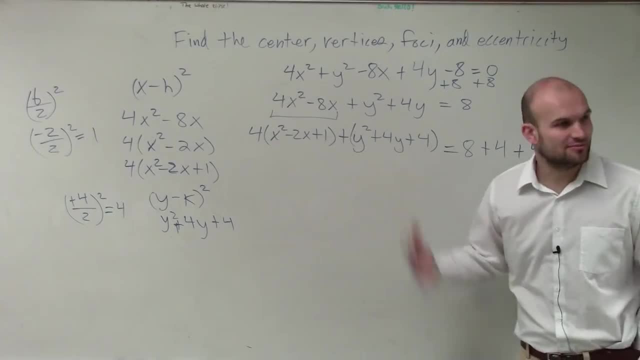 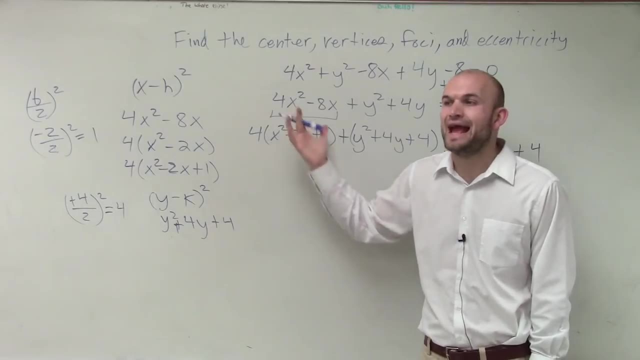 Yes, Okay. So now, why do we complete the square again? Why do we care that these are perfect square trinomials? The reason why we like perfect square trinomials and the reason why we have to complete the square to create perfect square trinomials. 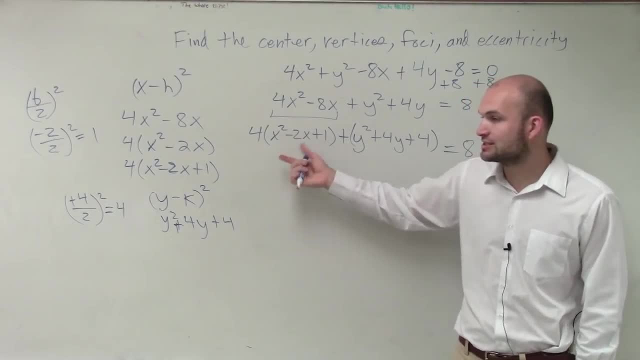 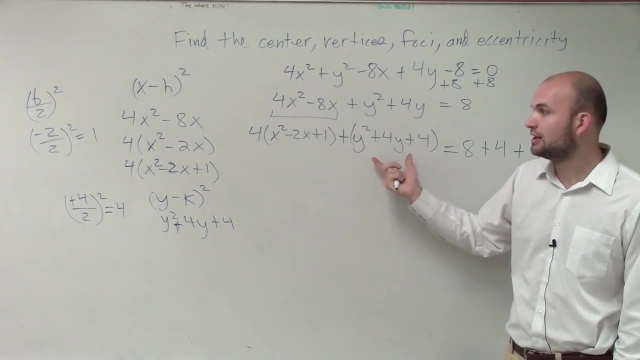 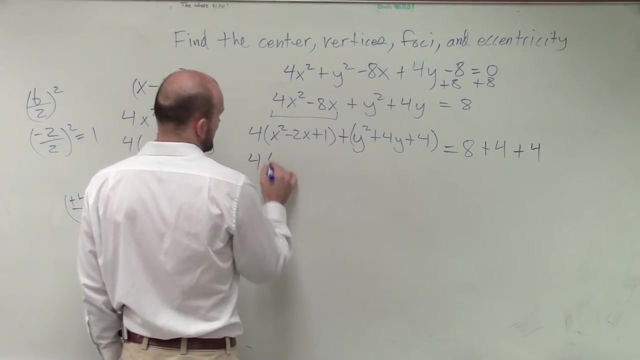 is because when we factor these, when I factor this, it creates a binomial square. When I factor this- because I completed the square to make it a perfect square, trinomial- its factored form is a binomial square, So let's go on to factor them to their binomial square. 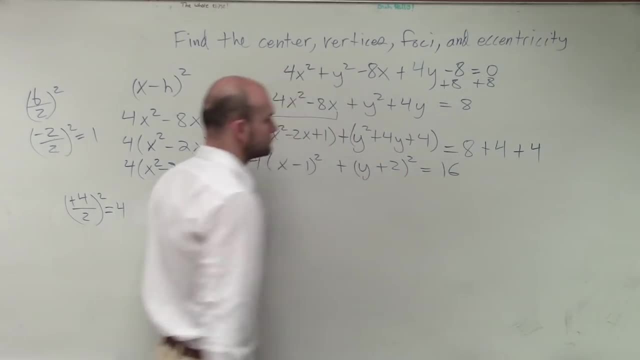 So we're almost there, right, Not looking too bad. However, we don't have an A inter B and we don't have it equal to 1.. So to make this equal to 1, I can divide by 16,, right. 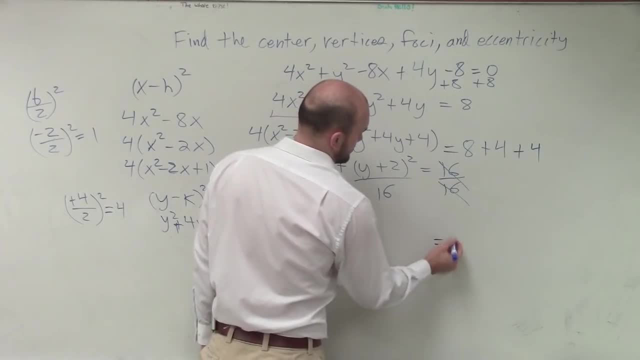 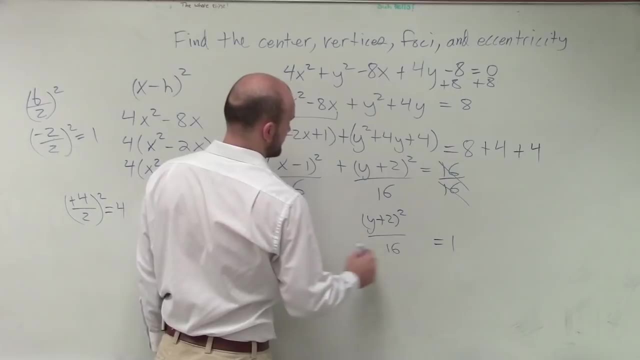 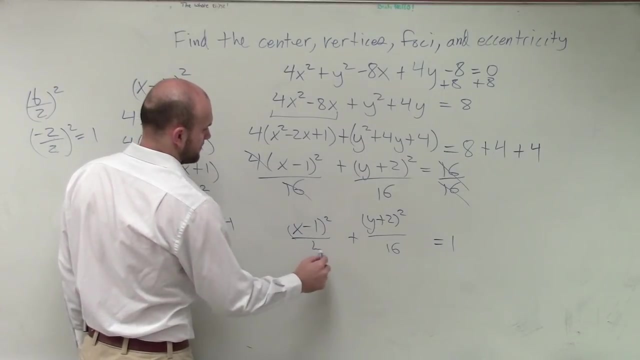 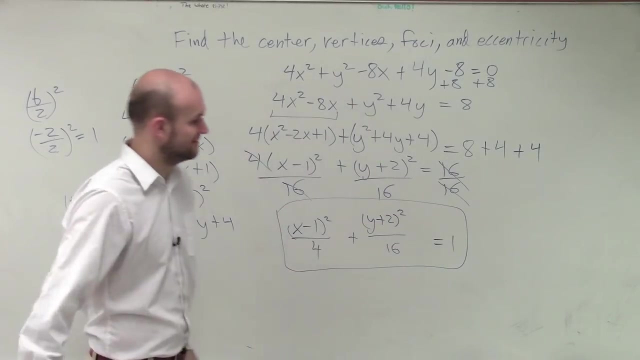 So we know now this. that goes to 1.. This is just going to remain the same. Y plus 2, squared over 16, plus this, reduces down to 1. fourth, Okay, So almost there. Alright. So now, ladies and gentlemen, we have it. 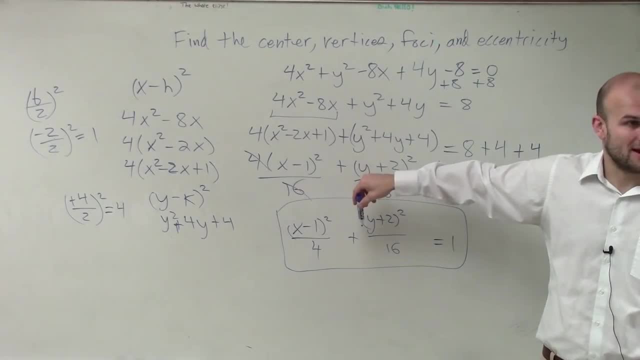 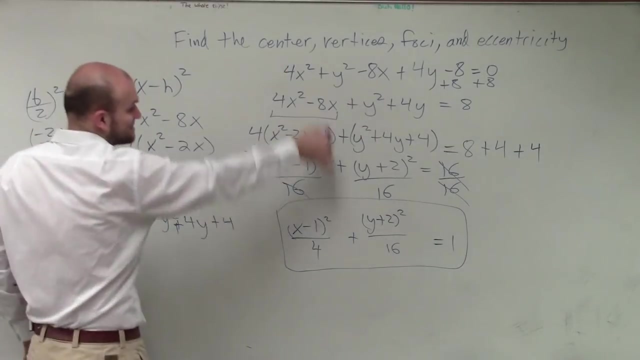 So we went from this to this right, This to this. Now it sends us in this form. They said: find the center. Can we easily find the center? The center is Negative 1, 2.. Close. Remember it's opposite of H, opposite of K. 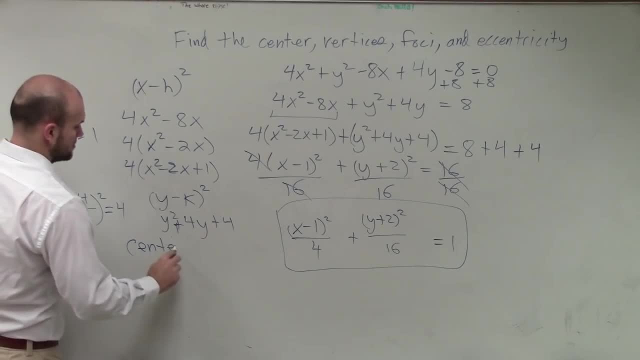 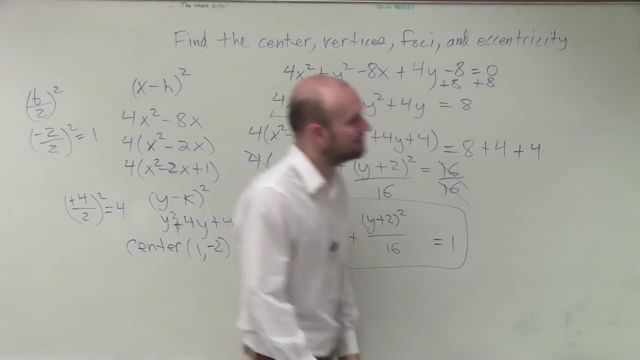 So the center is 2, 1.. 1, negative, 2.. Right 1, negative, 2.. You know, if you just keep on yelling out you'll get it. But yeah, just remember, it's the opposite of H and K, okay? 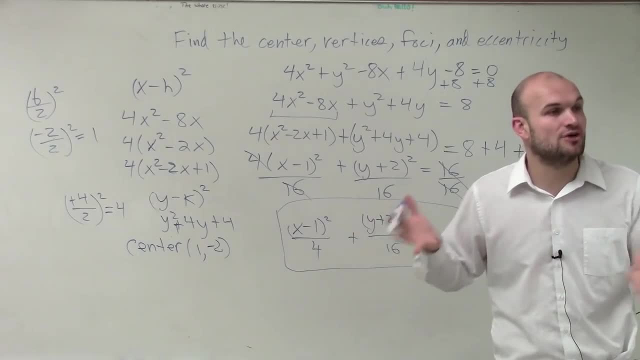 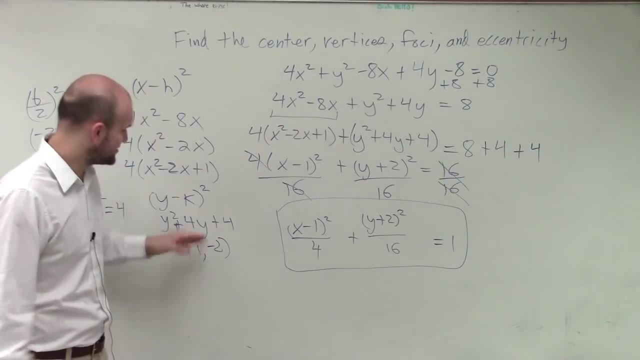 And remember, X is in the ellipses, X is always going to be with your H. Same thing with the parabolas, right? Yes, Good, Yes, okay, Good. So we have center equals 1, negative 2.. 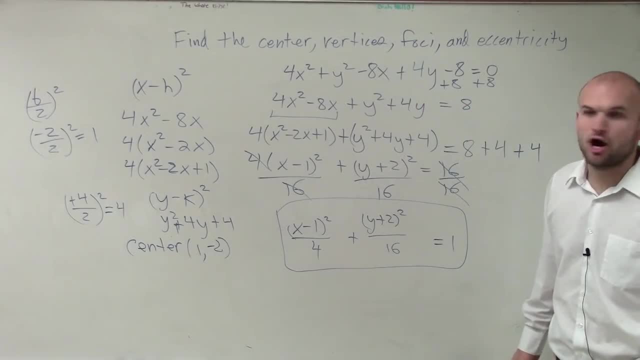 Then they say: find the vertices. Well, ladies and gentlemen, the vertices are: how far away from the center? 2, A, 2, I don't know really. 2, A, A, A. Okay, Let's stop, Let's take a break here. 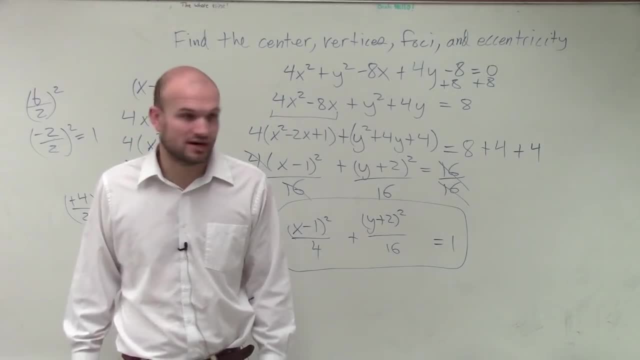 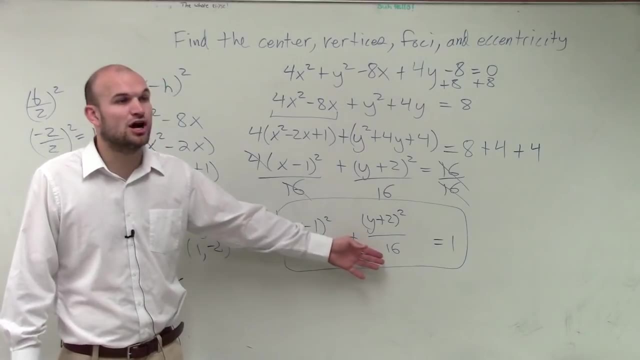 First thing we need to do, before we even start talking about vertices and foci, let's look at this graph. Is this graph going to be horizontal or vertical? Vertical? Vertical because our larger term, which is our A squared, is under the Y squared right. Alright? So now, ladies and gentlemen, we have it. 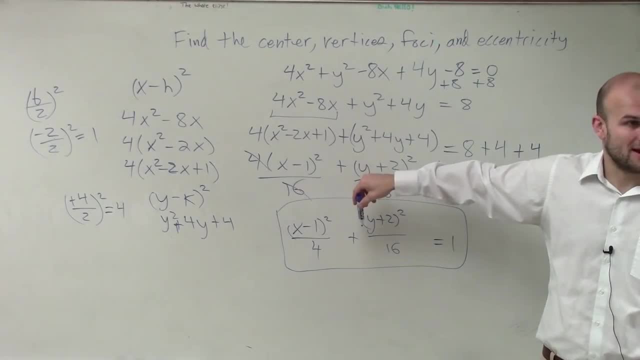 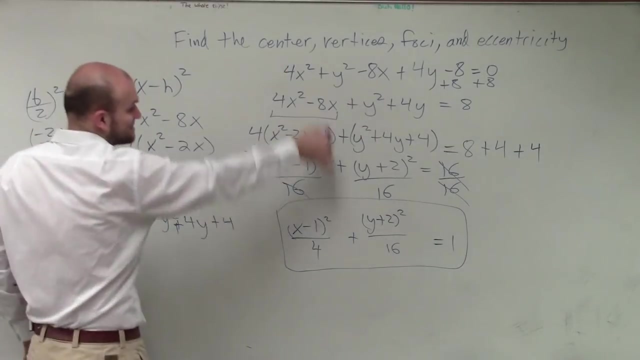 So we went from this to this, right? This to this. Now, it sends us in this form. They said find the center. Can we easily find the center? The center is? Negative 1, 2. Close. Remember, it's opposite of H, opposite of K. So the center is? 2, 1. 1, negative 2. Right. 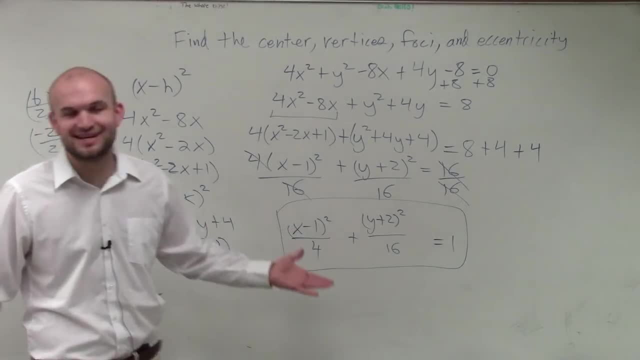 1, negative 2. You know, if you just keep on yelling out, you'll get it. 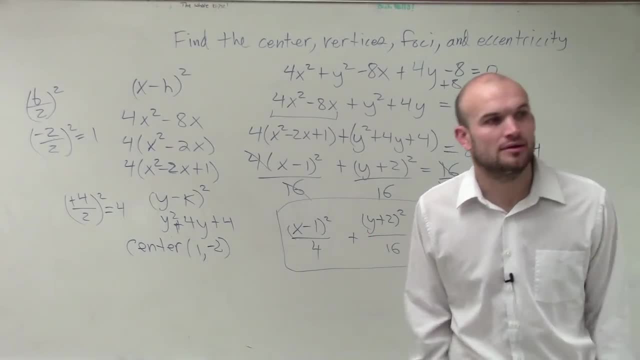 But yeah, just remember it's the opposite of H and K, okay? And remember, X is, in the ellipses, X is always going to be with your H. Same thing with the parabolas, right? Yes? Good. 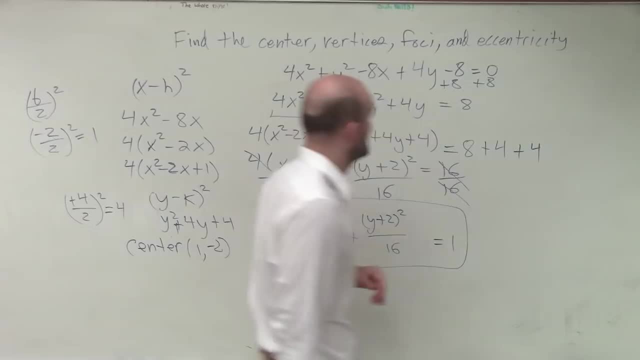 Yes, okay. Good. So we have center equals 1, negative 2. Then they say find the vertices. Well, ladies and gentlemen, the vertices are how far away from the center? 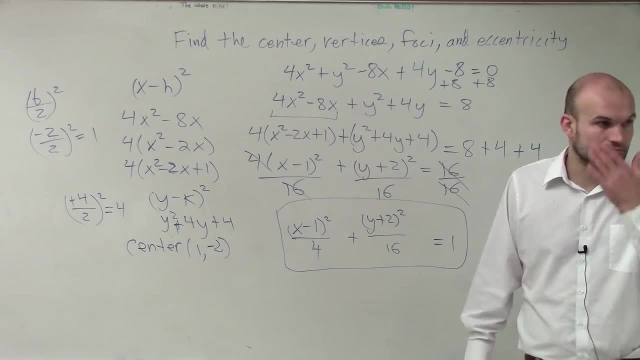 2, A. 2, I don't know, really. 2, A. A. A. Okay. Let's stop. Let's take a break here. 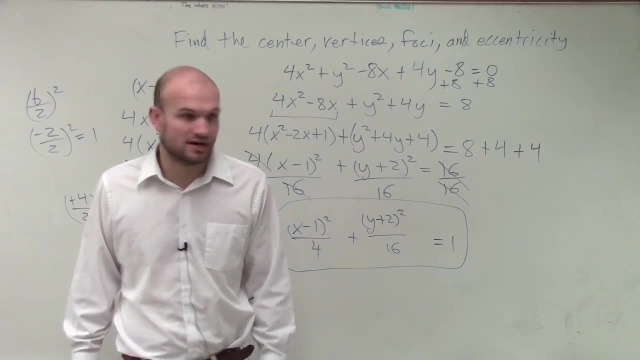 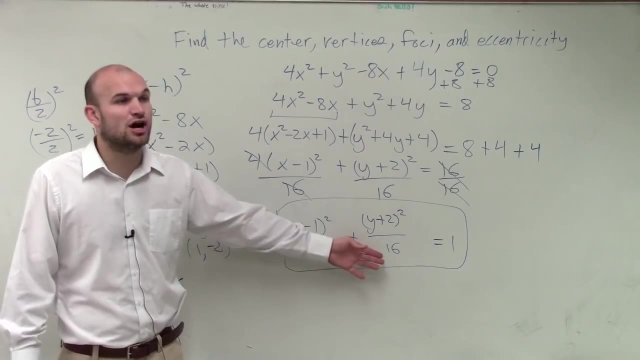 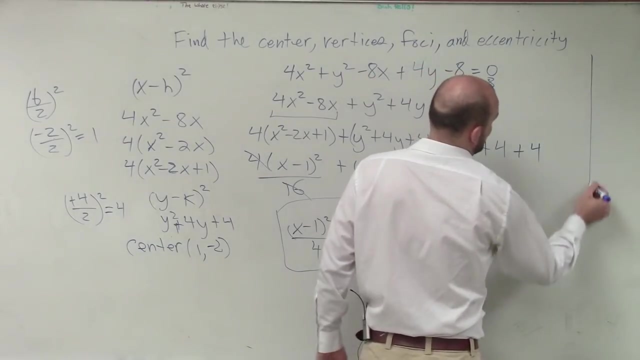 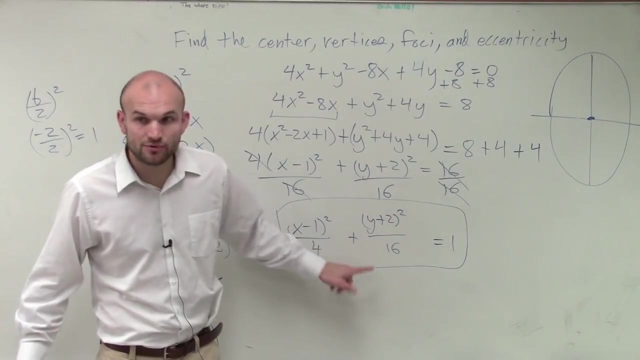 First thing we need to do, before we even start talking about vertices and foci, let's look at this graph. Is this graph going to be horizontal or vertical? Vertical. Vertical because our larger term, which is our A squared, is under the Y squared, right? So let's go and plot a graph of this real quick. It doesn't need to be pretty. So now we know, since it's a vertical, because my A squared is under my Y, I know that I have foci and vertices. 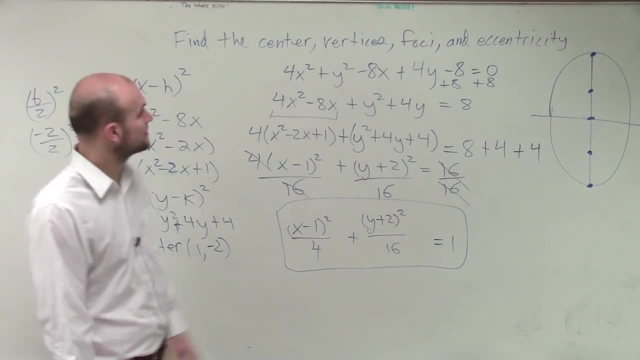 Now, we said the center is at 1, negative 2. 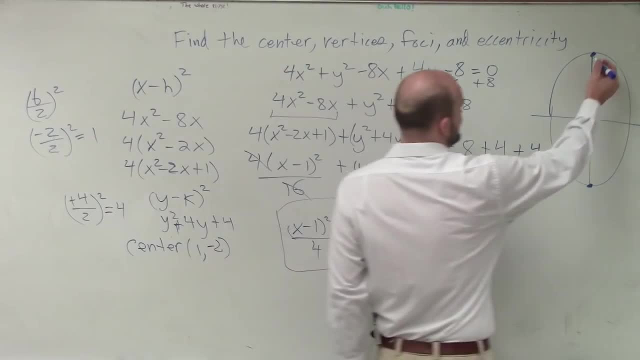 Let's go and determine what the vertices are. Now remember, this distance from the center to a vertices has a distance of A. 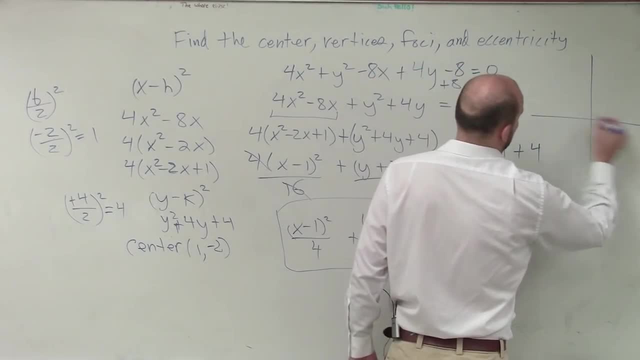 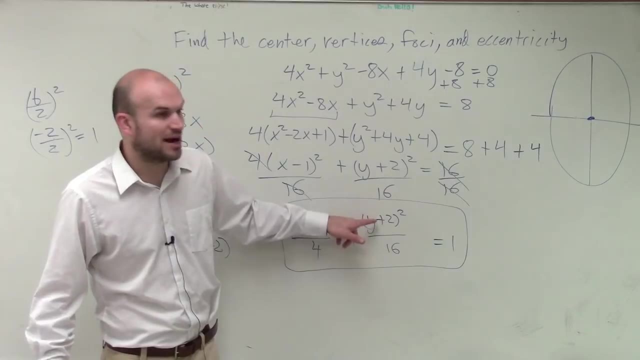 So let's go and plot a graph of this real quick. It doesn't need to be pretty. So now we know, since it's a vertical, because my A squared is under my Y, I know that I have foci and vertices. 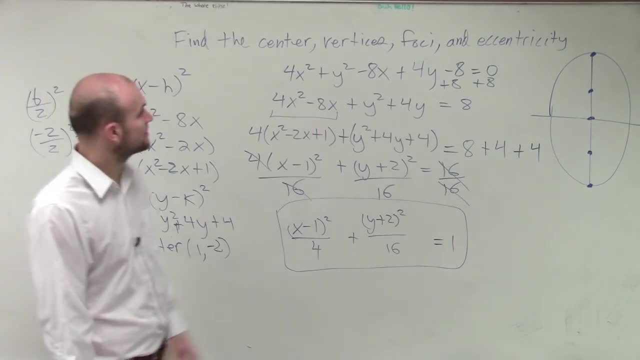 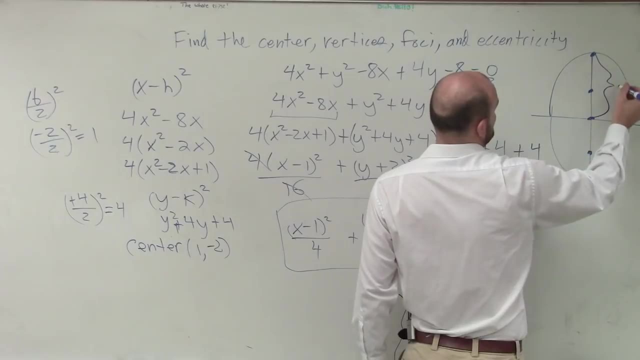 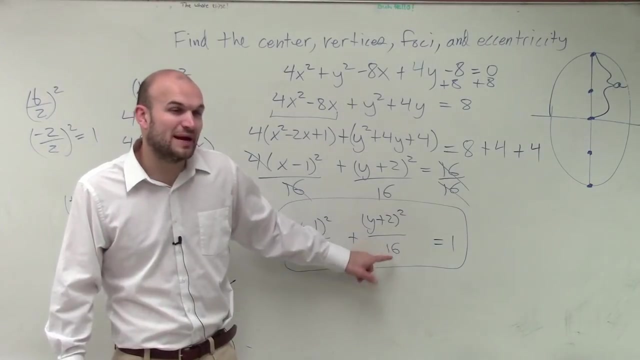 Now we said the center is at 1, negative 2.. Let's go and determine what the vertices are. Now, remember this distance from the center to a vertices has a distance of A And we're saying that A squared- remember A squared- is always your larger right. 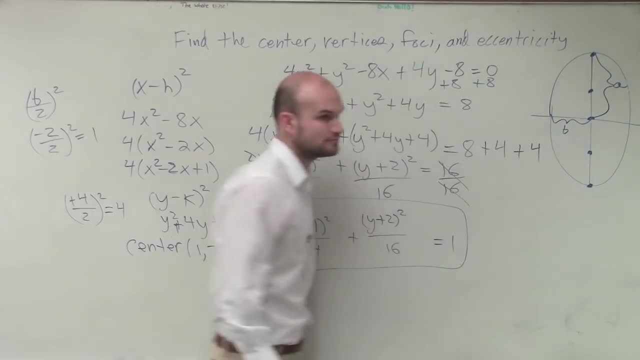 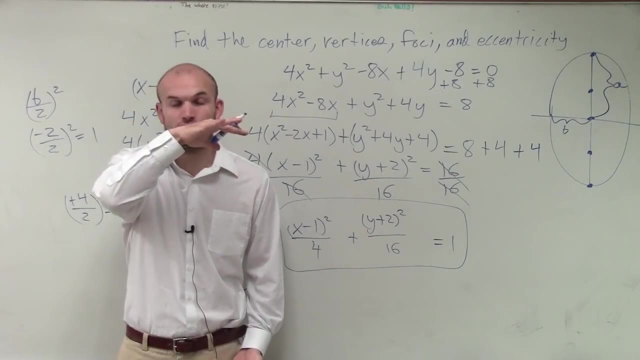 Because if this is A and that's B, right. So what we're saying is: your A squared, that's your larger one, since it's under the Y. that's what's made it vertical. So if I'm saying that 16 equals A squared, what is A? 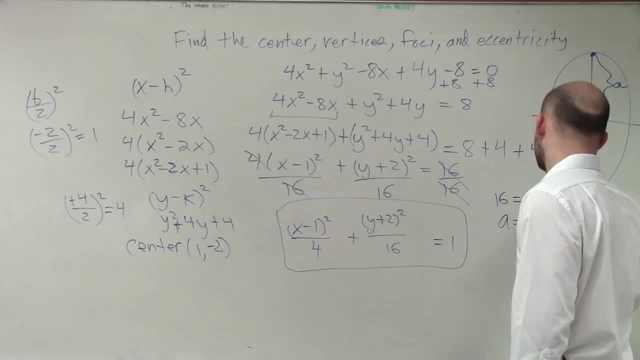 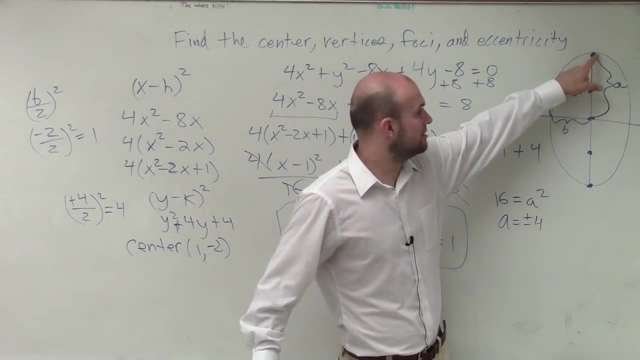 4.. 4, very good Plus or minus 4, though right, Because- notice, look at my center- I have to add 4 and I have to subtract 4,. right To get to my two vertices. I have to add and subtract. 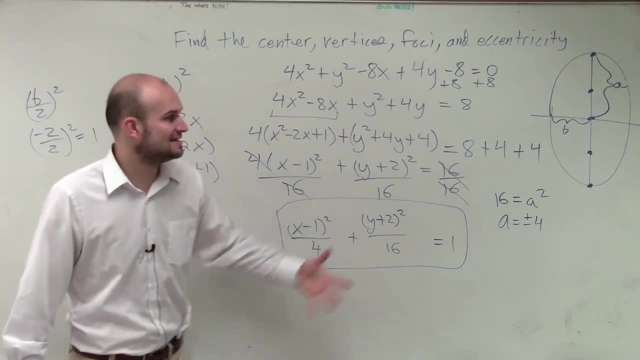 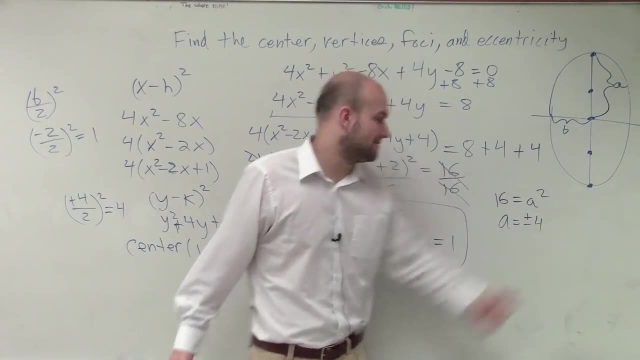 So it's plus or minus 4.. Now am I plus or minusing that to the H value or the K value of my vertex, The X or the Y, as you could say, The Y coordinate right, which is your K? 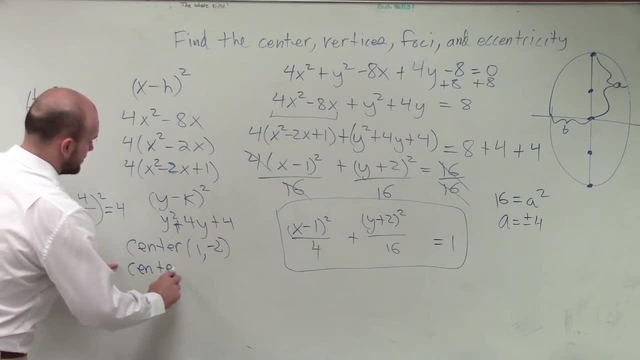 So, therefore, my center, 1.. 1.. 1 is going to remain the same, but it's going to be negative, 2 plus or minus 4.. Does that make sense? No, No, it really doesn't. The 1 remains the same. 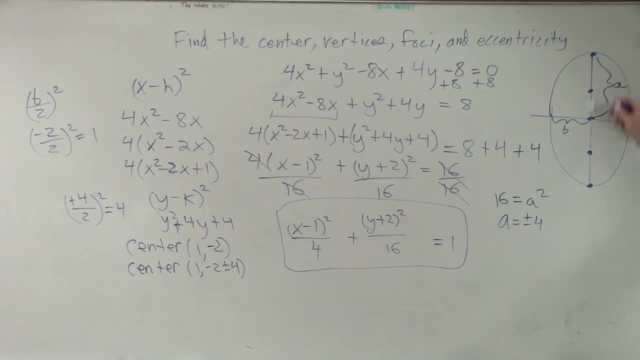 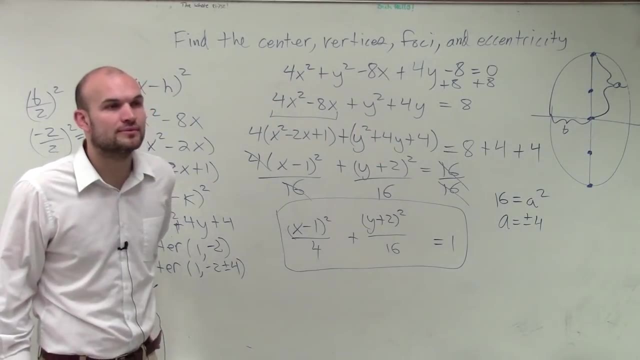 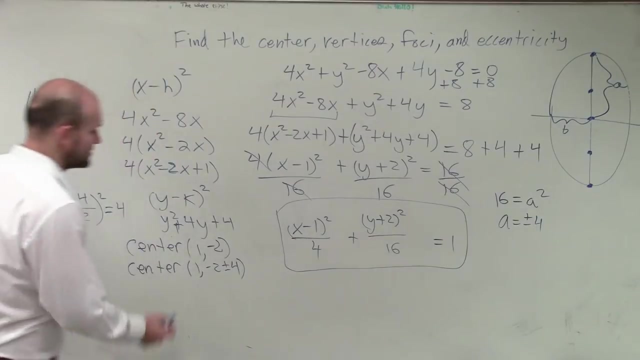 The center. the X value remains the same. They're all on the major axis. What's your question? I don't understand. Just keep going. I was in your last class. We can go right through it. We can go right through it. 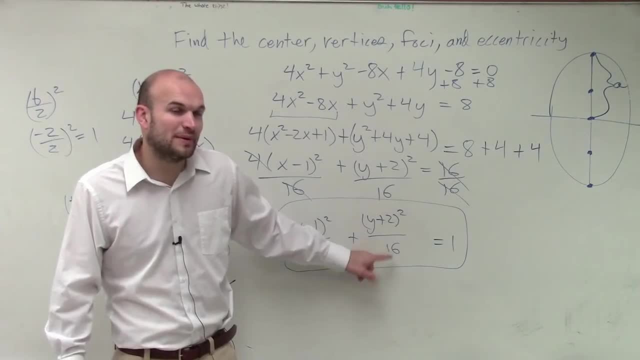 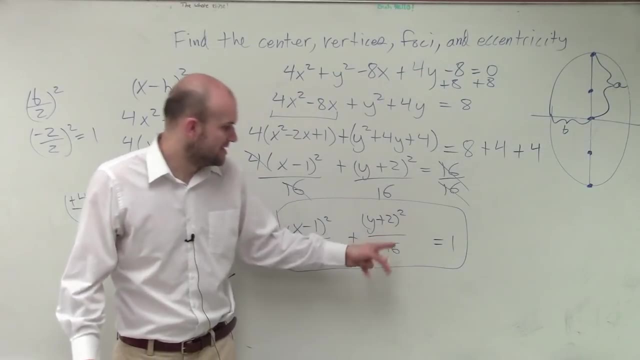 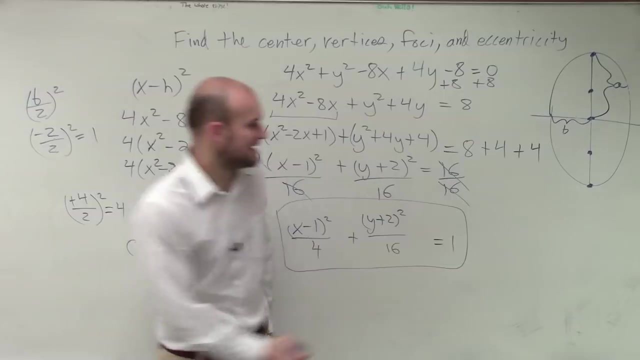 And we're saying that A squared, remember A squared is always your larger, right? Because if this is A and that's B, right? So what we're saying is your A squared, that's your larger one, since it's under the Y, that's what's made it vertical. So if I'm saying that 16 equals A squared, what is A? 4. 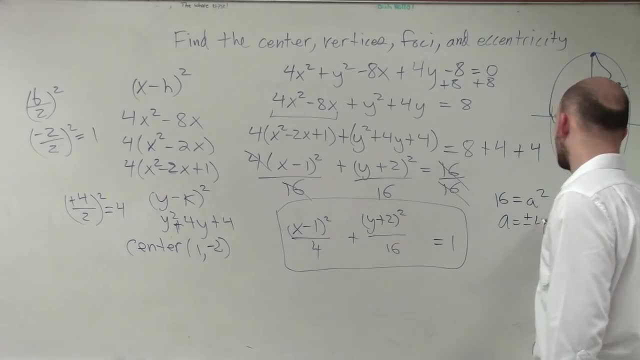 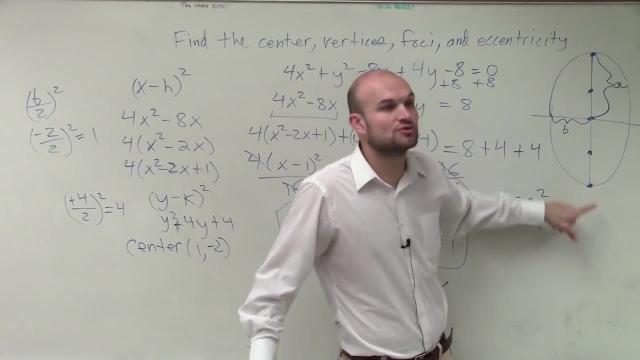 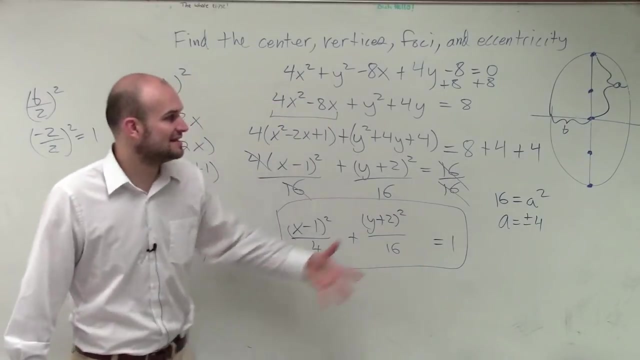 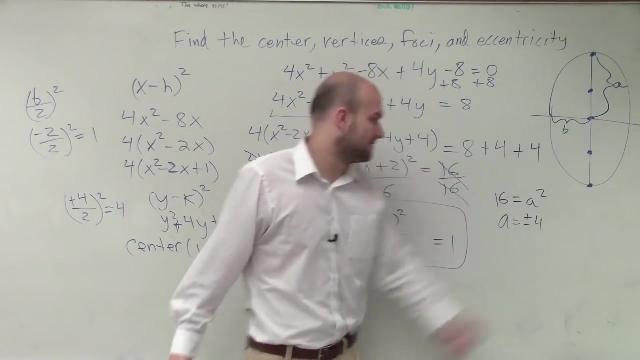 4, very good. Plus or minus 4, though, right? Because notice, look at my center. I have to add 4 and I have to subtract 4, right? To get to my two vertices, I have to add and subtract. So it's plus or minus 4. Now, am I plus or minusing that to the H value or the K value of my vertex? The X or the Y, as you could say. The Y coordinate, right, which is your K. 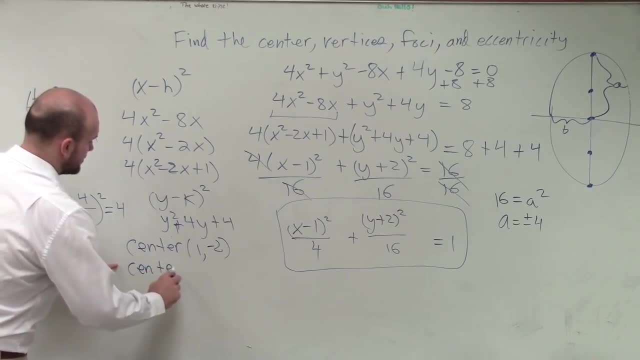 So therefore, my center... 1. 1. 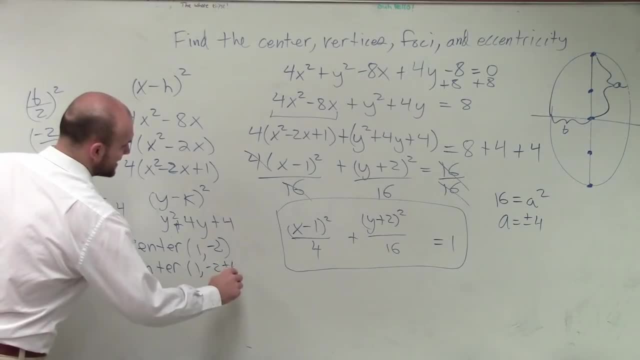 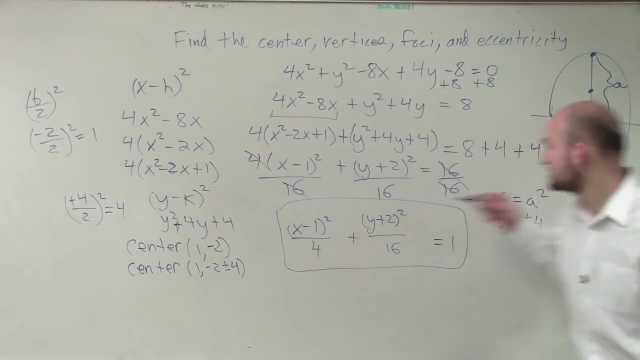 1 is going to remain the same, but it's going to be negative 2 plus or minus 4. Does that make sense? No. No, it really doesn't. The 1 remains the same. The center, the X value remains the same. 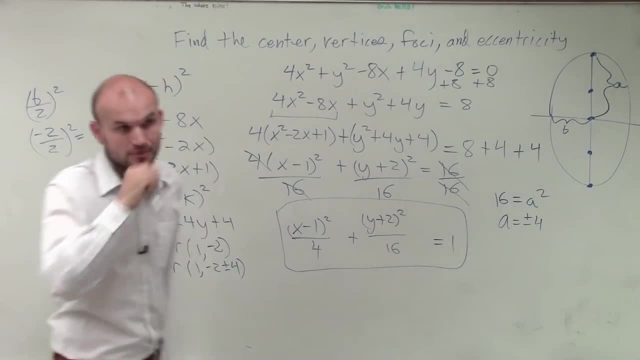 They're all on the major axis. What's your question? I don't understand. Just keep going. 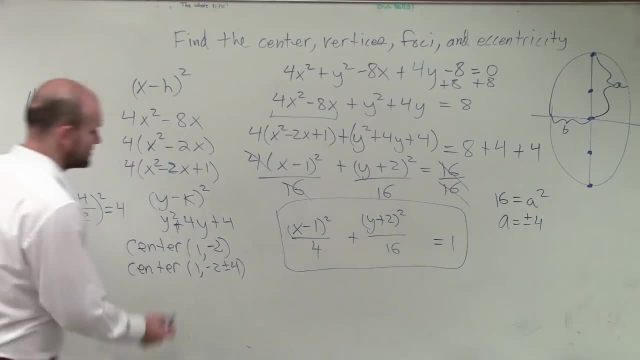 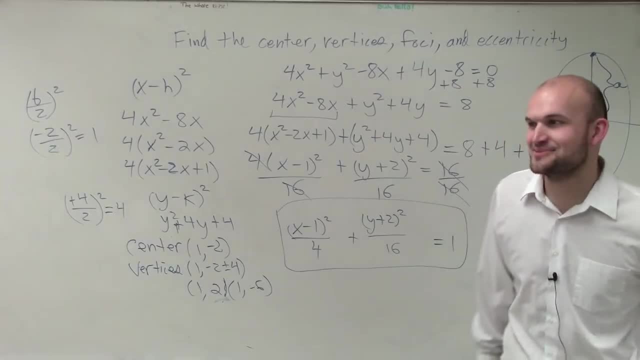 I don't care. 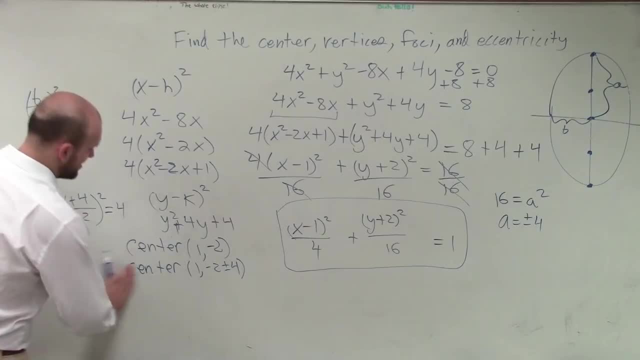 So therefore we have our center is officially going to be at. I'm sorry, your ver. Oh, why am I rewriting this? Yeah, that's what I was. No wonder you're not making sense. We see you. I don't know what you're doing. 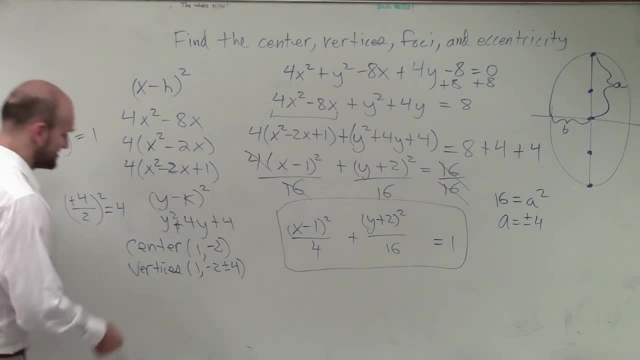 Oh, right in the sentence. So your vertices are going to be at: 1 comma 2.. 1 comma 2 and 1 from the negative 6.. 1 comma, negative 6.. How about I just write: everything is labeled a center, and then you guys can just guess. 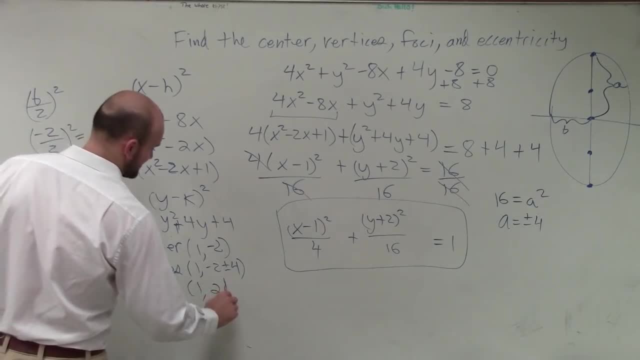 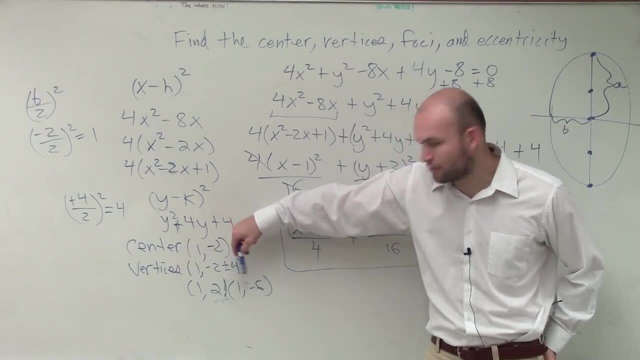 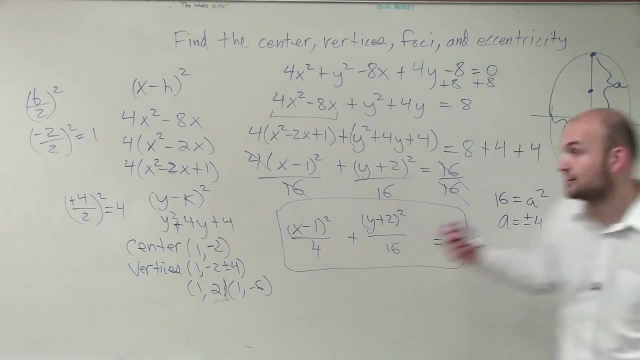 So now in the sentence we have 2 vertices Right. Your vertices is 1 comma 2 and 1 comma negative 6. Notice how they all have your center and your vertices. all have the same x coordinate Right Because they all lie on the major axis. 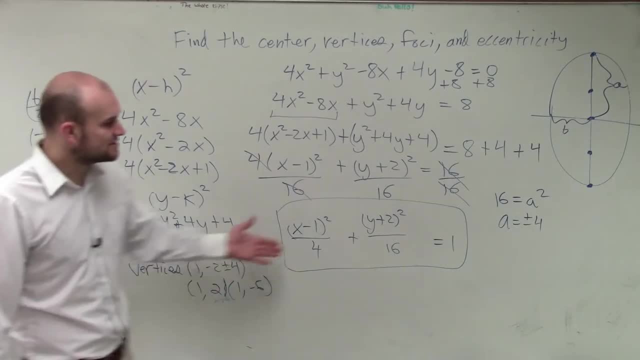 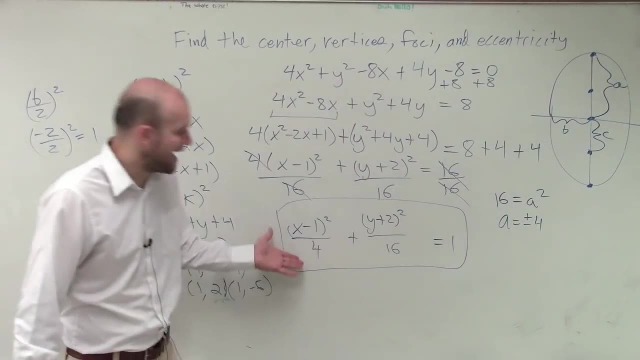 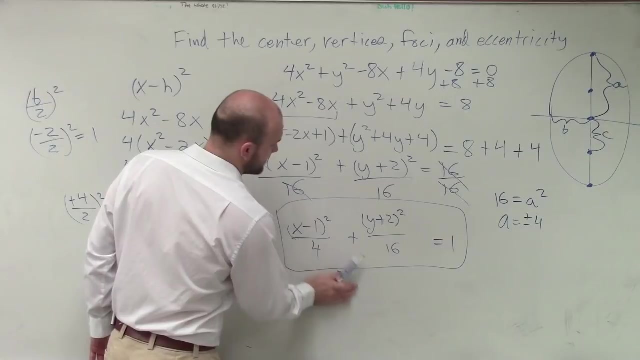 Last thing we need to do is find the foci. Well, ladies and gentlemen, foci has a distance of c, And we got a little issue with that, because do we have a c in this formula? No, No, is a squared equals b squared plus c squared right. 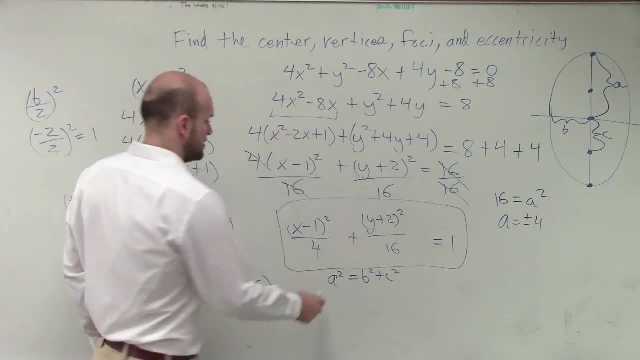 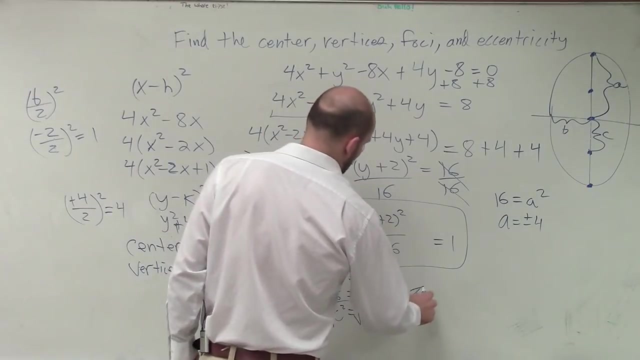 And do we know what a and b are? Yes, a is 16 equals 4 plus c squared. So by doing a little bit of work we can say c squared equals 12.. Take the root of both sides and I can say c equals the square root of 12.. 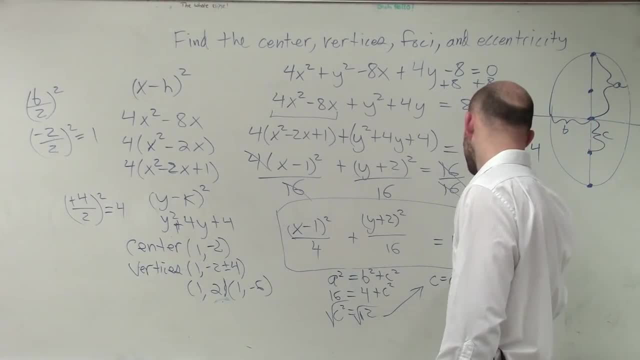 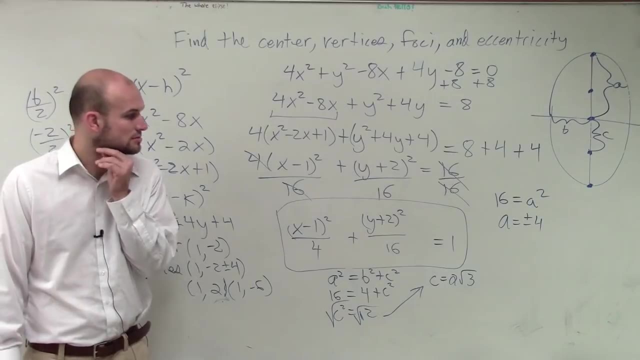 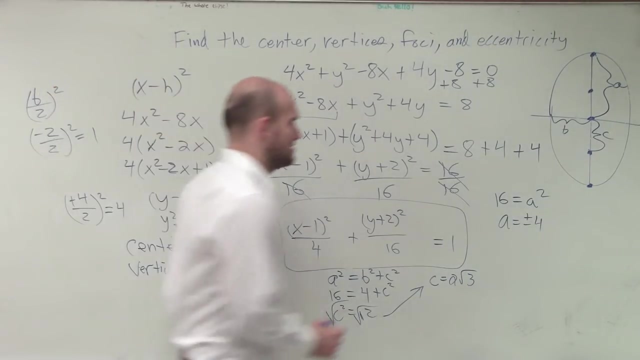 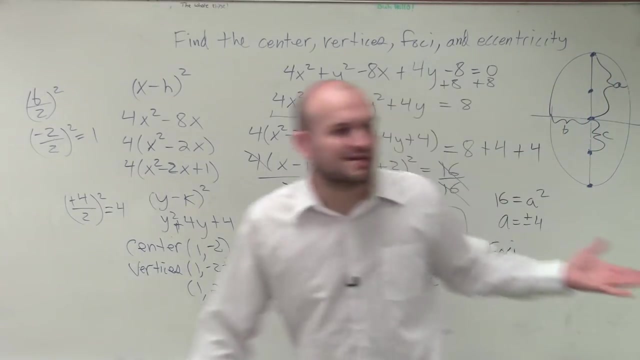 We can reduce that down to 2 radical 3.. Plus b: Huh, Plus b, Yes. OK, so I'll finish my work over here. So we have the center of the vertices. Now to find the foci. the foci is going to have the exact same x. 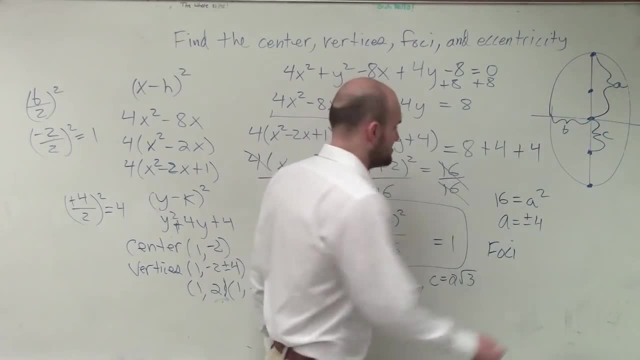 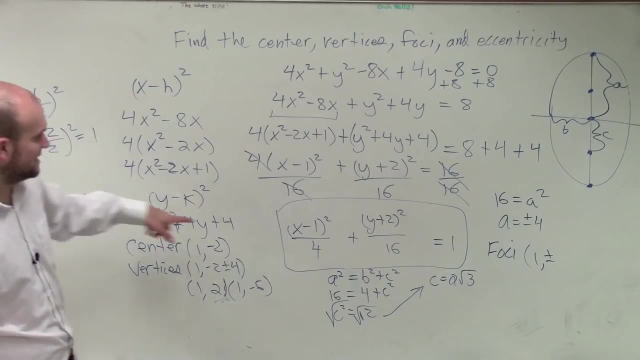 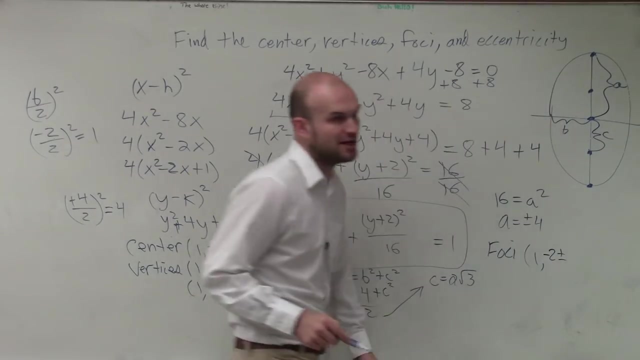 coordinate as the center and the vertices. Yes, Yeah, so we know it's going to be 1, right, 1 comma plus or minus the vertices, or the center, which is negative, 2.. Negative, 2 plus or minus. what's my value of c? I don't care. You got vertices, you've got vertices. You have two vertices. Right? 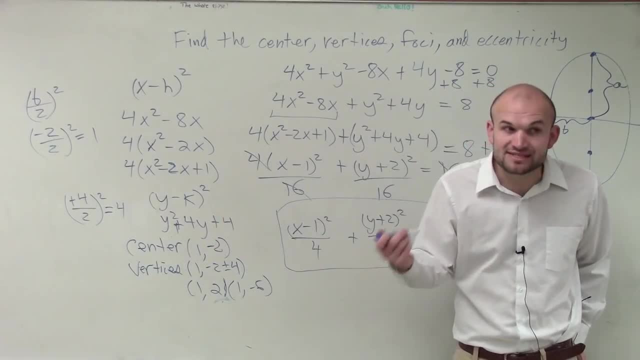 Your vertices is 1 comma 2, and 1 comma negative 6. Notice how they all have, your center and your vertices, all have the same x coordinate. Right? Because they all lie on the major axis. 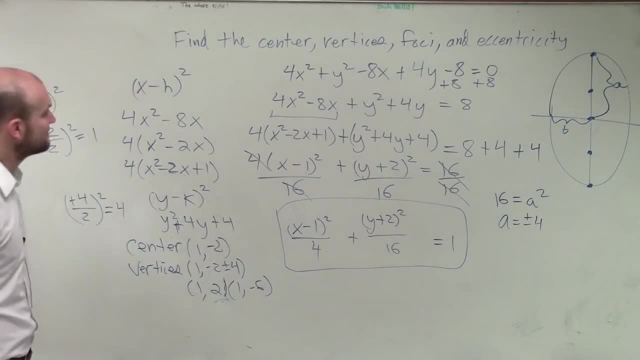 Last thing we need to do is find the foci. 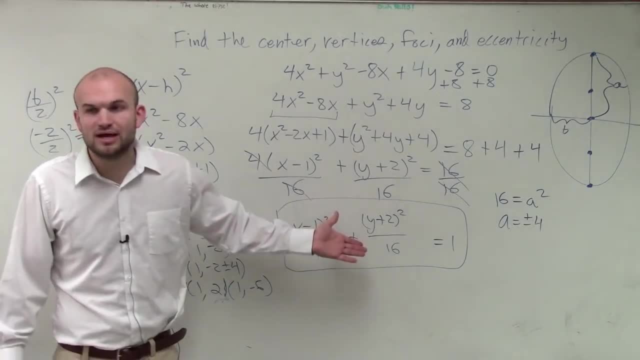 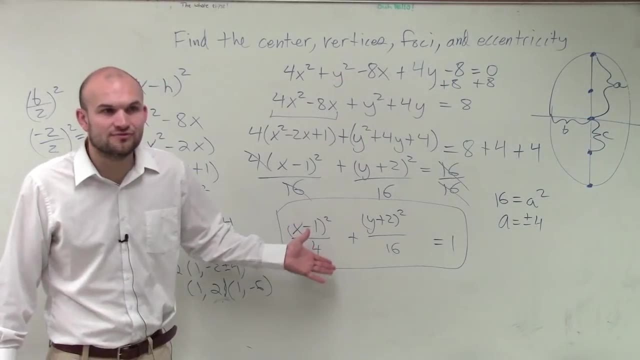 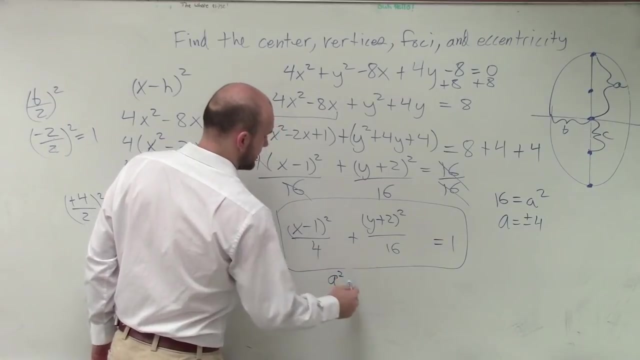 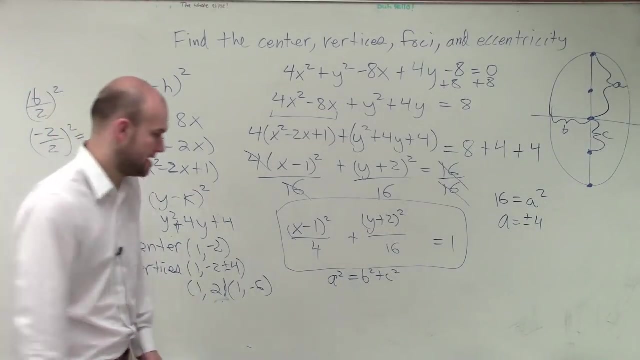 Well ladies and gentlemen, the foci has a distance of c. And we got a little issue with that, because, do we have a c in this formula? No. The only thing we do know is a squared equals b squared plus c squared. Right? And do we know what a and b are? Yes. a is 16 equals 4 plus c squared. So by doing a little bit of work, we could say c squared equals 12. 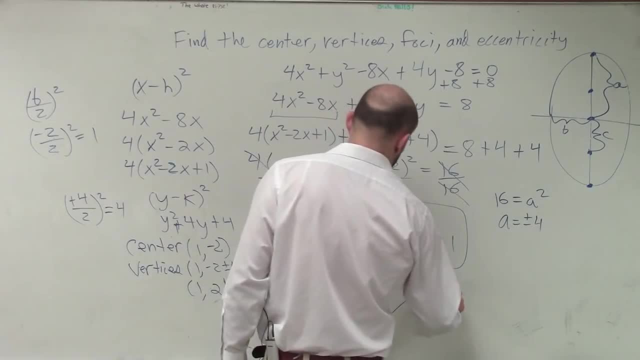 Take the root of both sides. And I could say c equals the square root of 12. 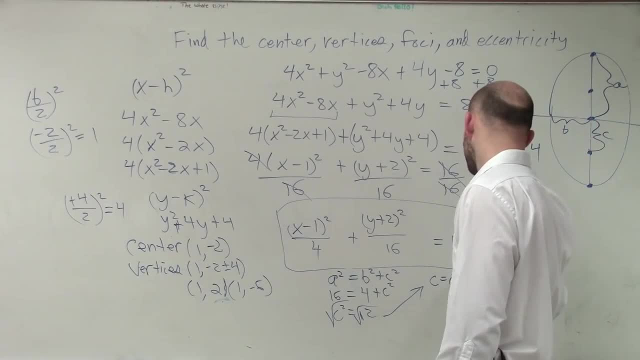 We can reduce that down to 2 radical 3. 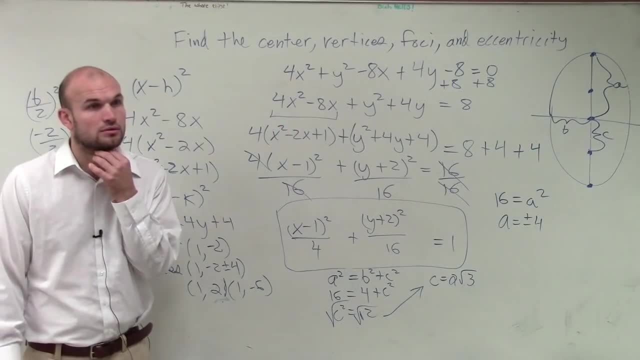 Plus b. Huh? Plus b. Yes. 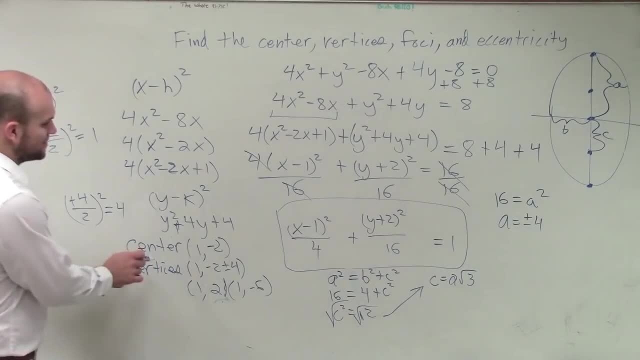 OK, so I'll finish my work over here. So we have the center of the vertices. 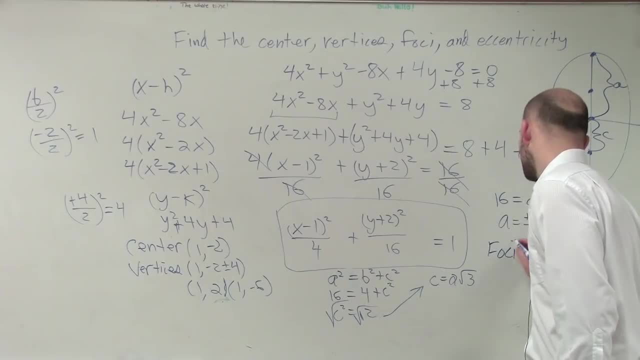 Now to find the foci, the foci is going to have the exact same x 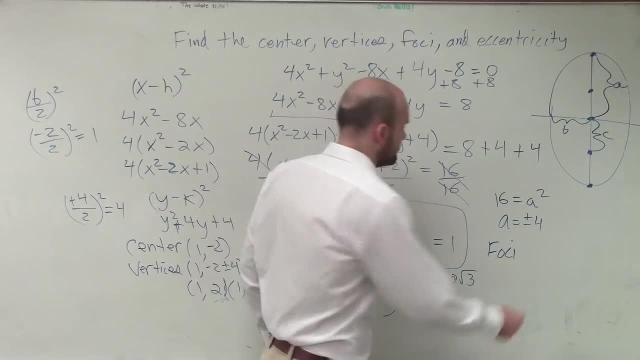 coordinate as the center and the vertex. The vertices? Yes. Yeah. So we know it's going to be 1, right? 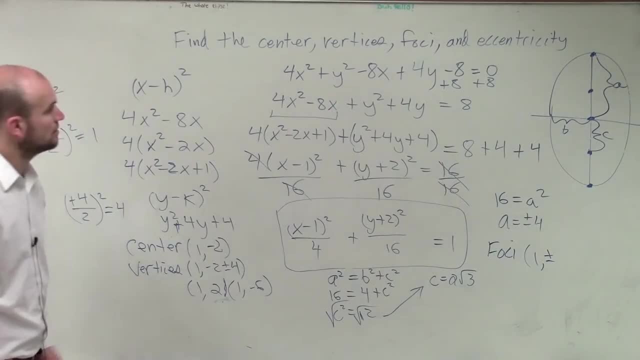 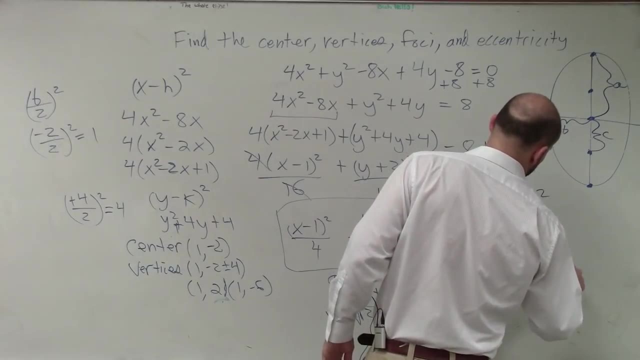 1 comma plus or minus the vertice or the center, which is negative 2. Negative 2 plus or minus, what's my value of c? 2 square root of 3. 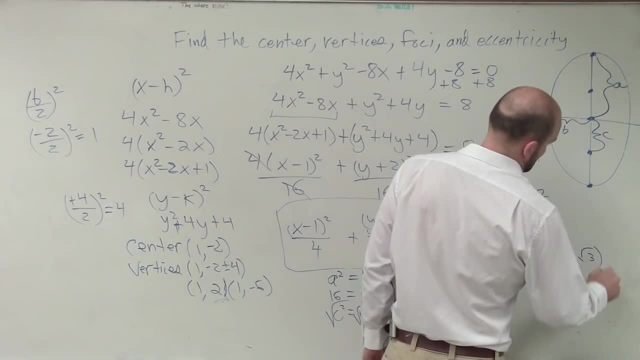 2 square root of 3. Now, can we add a 2 square root of 3 to a negative 2? No. 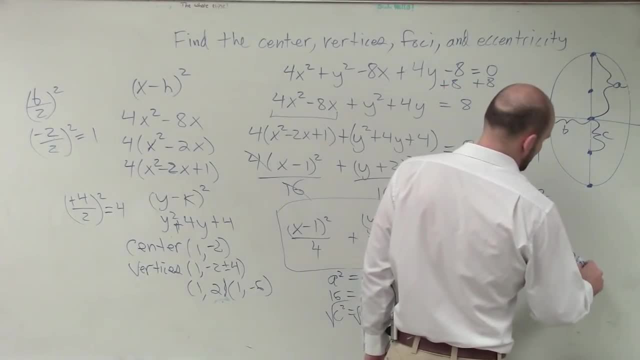 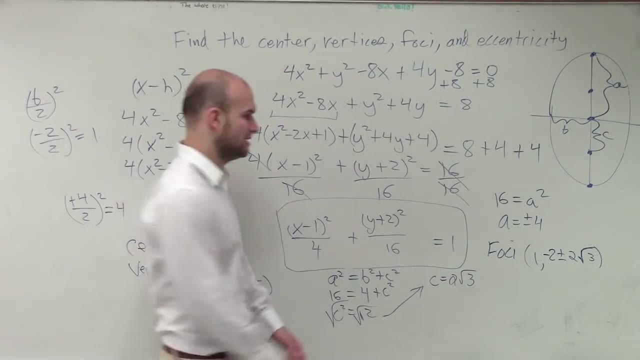 2 squared of 3.. 2 squared of 3.. Now can we add a 2 squared of 3 to a negative 2? No, No, So we can just write our quote, guys, As 1 comma negative 2 plus 2 squared of 3.. 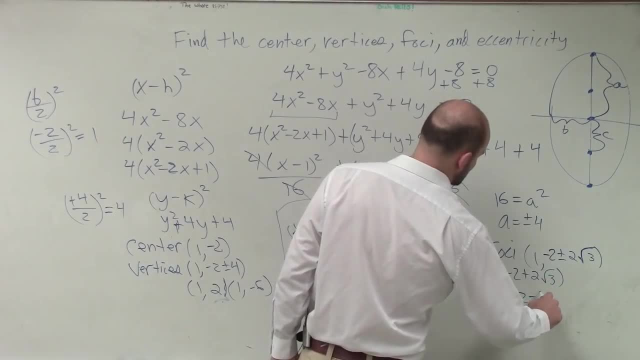 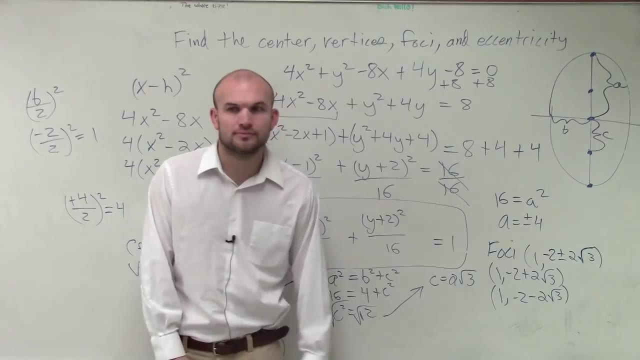 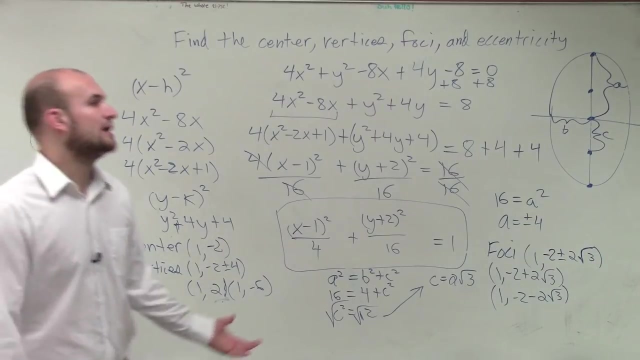 And our other foci is 1 comma negative 2 minus 2 squared of 3.. Do not leave me a decimal form. Leave this in an exact form, all right. So now we have our foci center and our vertices. 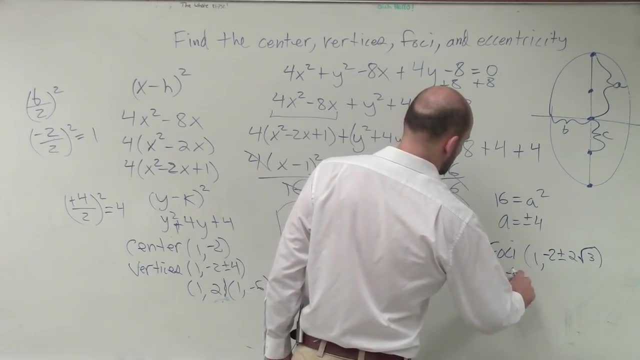 So we can just write our quote, guys. 4 squared. As 1 comma negative 2 plus 2 square root of 3. 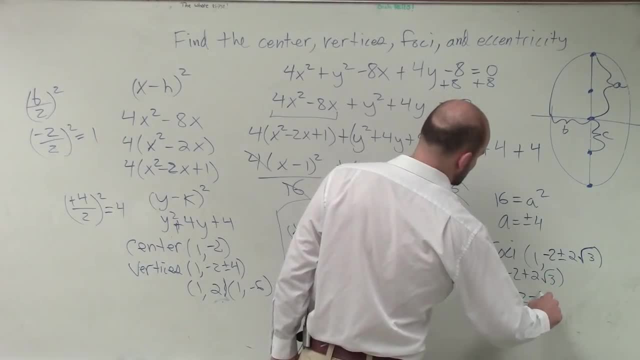 And our other foci is 1 comma negative 2 minus 2 square root of 3. Do not leave me a decimal form. 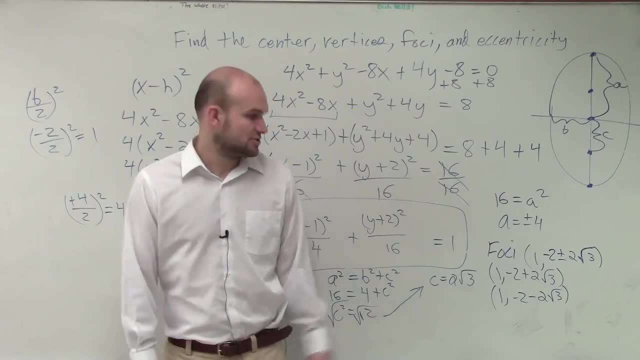 Leave this in an exact form. All right?